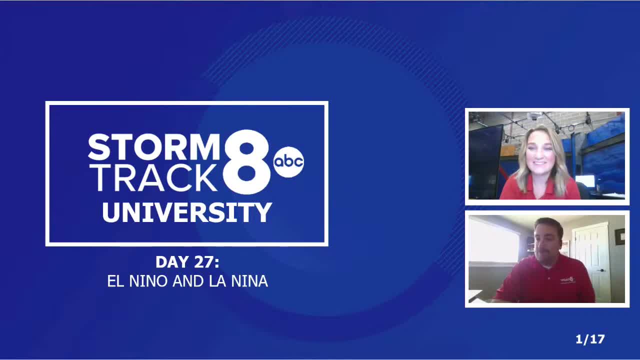 did kind of overshoot last week. We held you back about seven, eight minutes, I think it was, So we'll get you a little early out today. But as always, if you have questions whether it's today's lesson, any other lesson, feel free to go ahead and put those in the comments section. 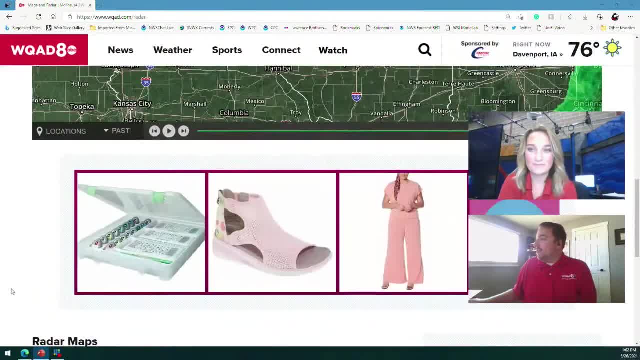 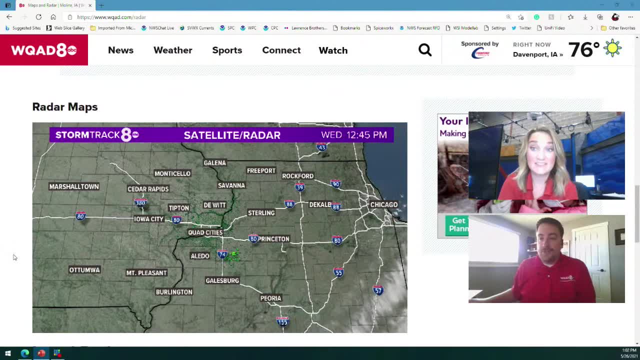 And we'll get to those here right at the end. Let's start with what's going on outside. I was looking at the radar. a whole lot of nothing, In fact. the clouds from this cold front that moved through very early this morning, now moving out of the region. 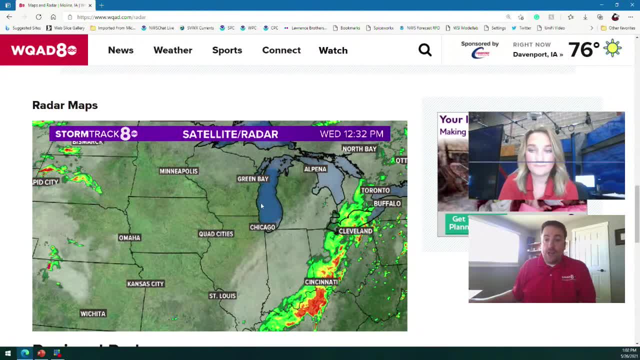 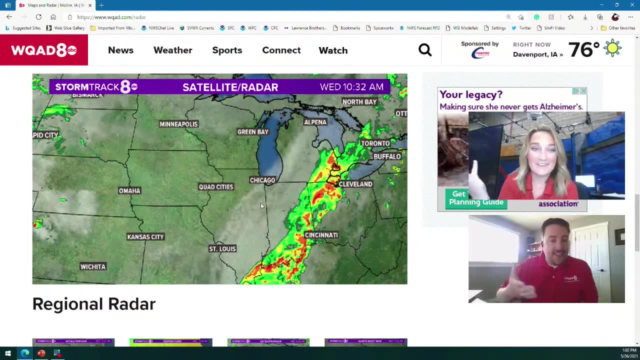 There you can see the complex of showers and storms that we had this morning. It came in here in Geneseo around four o'clock A little bit of a wake up, with a few bolts of lightning and some heavy rain. Did you hear anything? 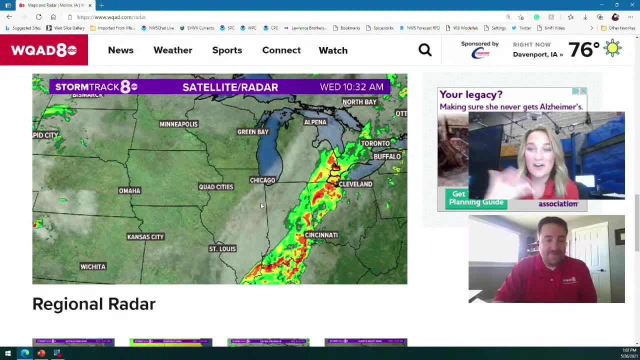 Nope, I didn't even know it rained until I woke up and I just saw some posts about rain. I went outside. My car was still wet. I was like, oh, I guess it rained. Yeah, it came in so late And, all honestly, before I went to bed I looked at the radar. 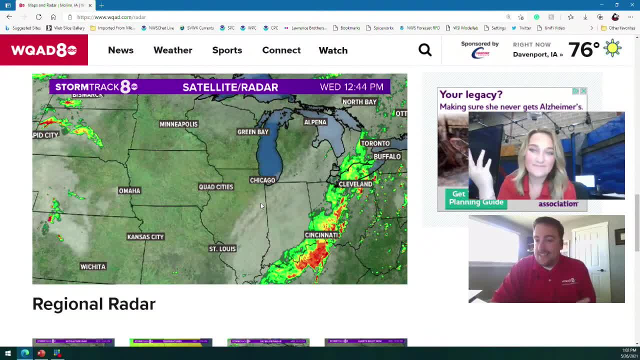 the stuff in Iowa was falling apart. It's like we're not going to get anything. This is another dud. But it actually did develop a little complex to the west of Quad Cities And that moved in really late last night. First I thought it was dreamy because we have not heard thunder very often this year so far. 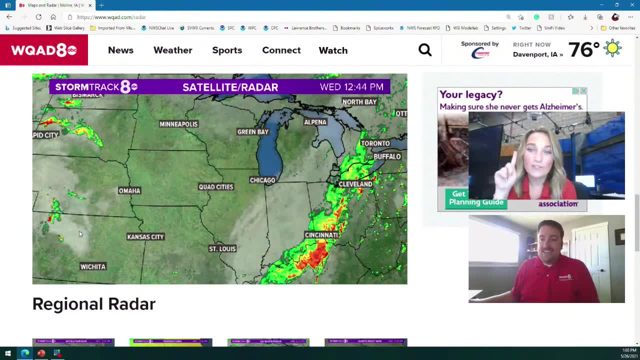 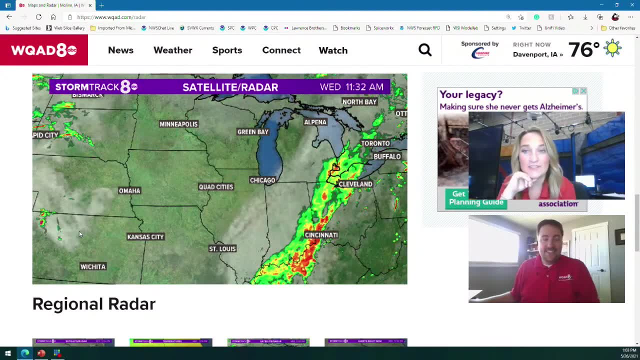 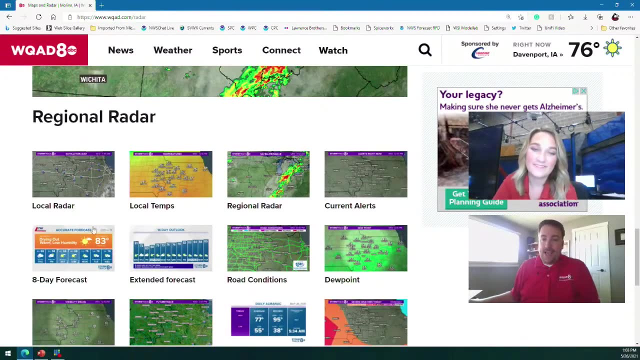 This is a little nice. Heard it twice, Isn't that sad? And only I've only heard it twice, and only one, one crack of thunder, which with each storm, So it wasn't even exciting, It was just once. Yeah, it's just been so lackluster this year. We'll see if things can pick up here in the near. 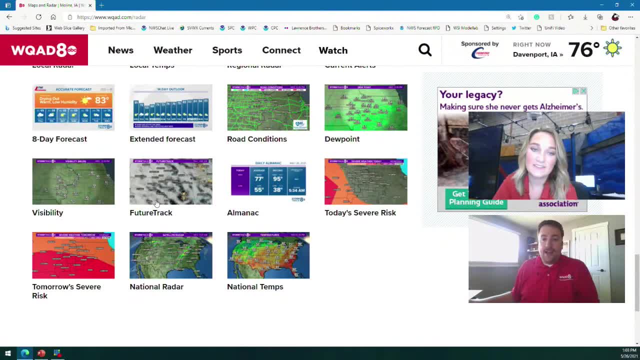 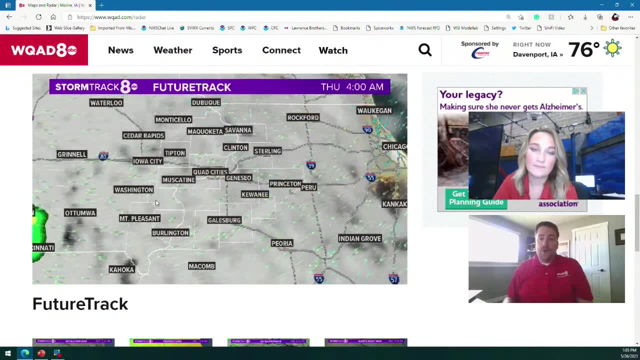 term. I want to talk about what may potentially happen tomorrow And I'll go through a future track really quickly for you here This afternoon. this evening is pretty quiet Getting through late tonight. more clouds coming in from the west. We'll watch. tomorrow There may be a complex of showers and storms in the 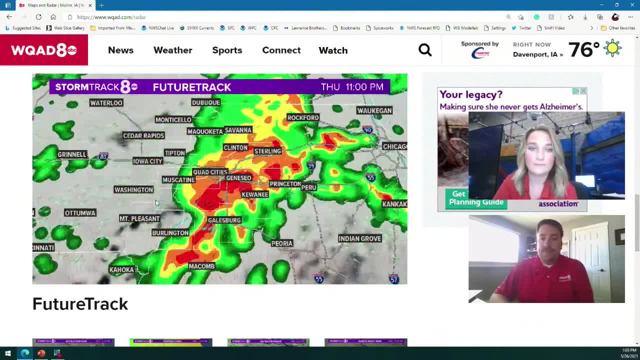 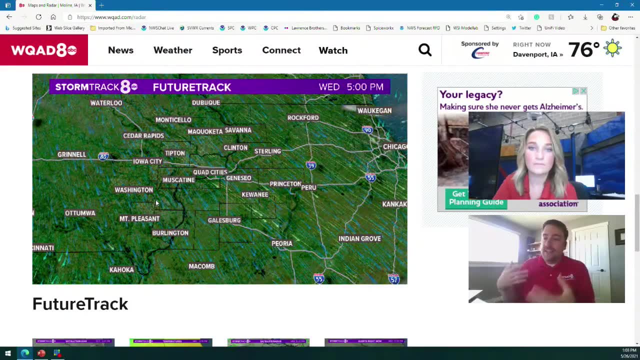 morning And then, depending on what happens with that, in the afternoon and evening, we may be looking at a stronger complex coming in mainly after the six, seven o'clock hour. tomorrow is very conditional, And that is really going to determine how much instability we can drive during the 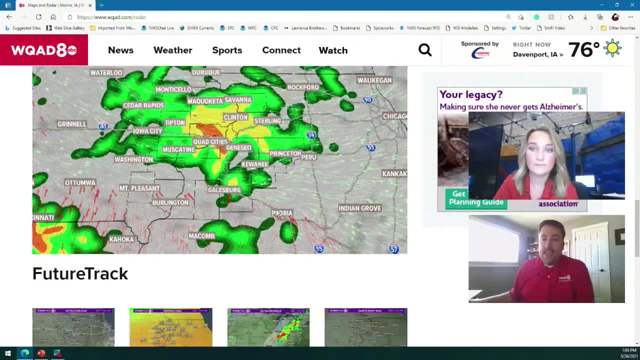 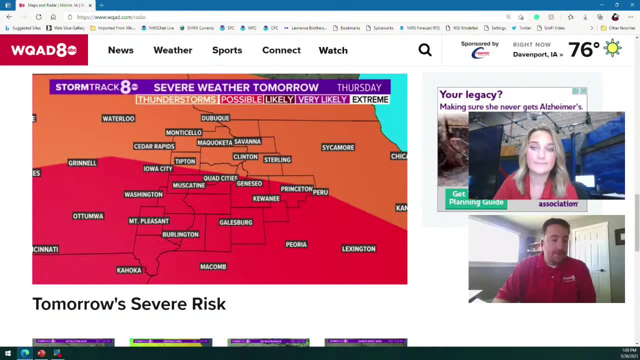 afternoon. You can see future track is fairly cloudy for much of the day, But I do want to kind of take note that the latest severe weather outlook, anyway, has nudged things a little bit further north in our direction. I'm just thinking of something really quickly because this may not have updated yet, But just 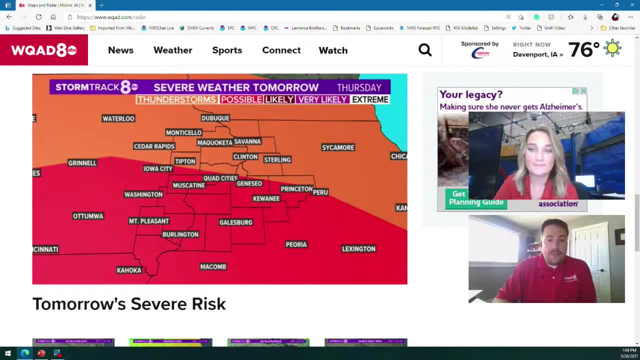 looking at the newer outlook that came out about half an hour ago, they've shoved the slight risk, which would be the darker red when this map will update here within the next hour or so. The likely category has now been shoved up to interstate 80. So those of you that are south of the quantities tomorrow, you're. 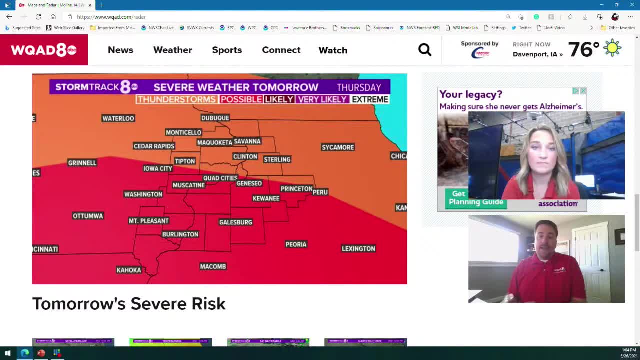 under that higher risk for some stronger storms. looking at mainly damaging winds, perhaps an isolated tornado as well. I see the tornado threat has moved up a little bit further to the north to mainly encompassing extreme southeast Iowa and west central Illinois in the higher tornado probability. 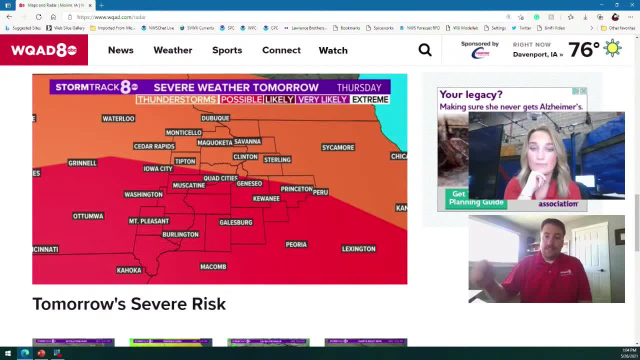 So keep an eye on that. You'll want to tune in to the forecast later tonight, especially the 10, and then Eric Sorensen tomorrow morning, because that will give us more information in terms of what may play out here For our severe weather chances tomorrow and maybe, if things play out just right, we might have a beast day and 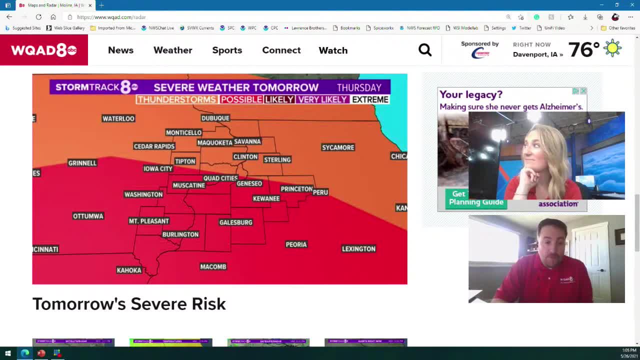 James is off tomorrow. I'm in the hot seat for him. So hopefully, if we do do that, Morgan, it's all you, It will be all me, So we'll keep an eye out on that. Yeah, hopefully we can get something out of that. I know that you've been dying to get in the beast for the 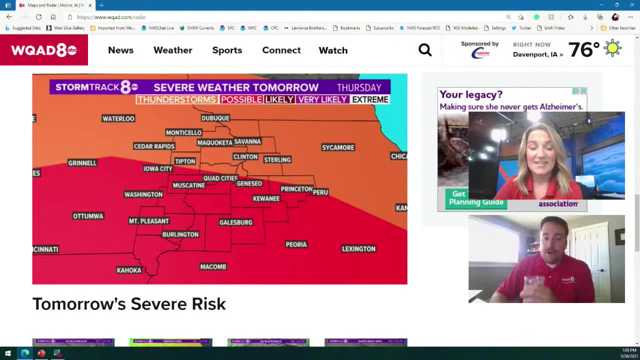 longest time, and tomorrow just might be that day. So we'll keep our eyes on that potential and see if it pans out. So again, watch this. We are watching tomorrow afternoon, tomorrow evening. A lot is going to depend on if we get who's son or. 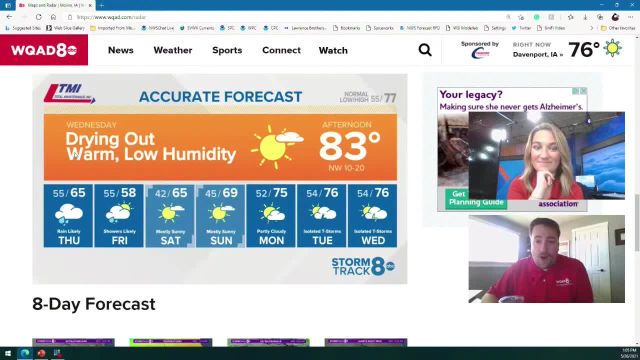 that. there's the rest of the forecast, though. Cool Friday, Oh my goodness. On the upper fifties we can turn the air off for not only Friday, but also Saturday, And of Sunday as well, And it looks like next week. 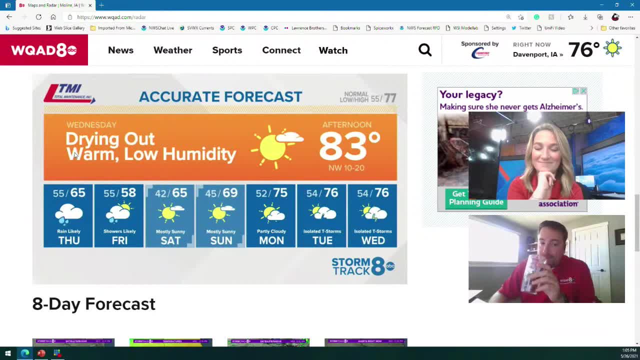 we can keep the air off. Any idea what might be happening behind? I have. It always happens nothing. nothing goes on. It's quiet it. and then the second you have something to do. i don't know what they're doing. one is ripping a paper into a thousand pieces. 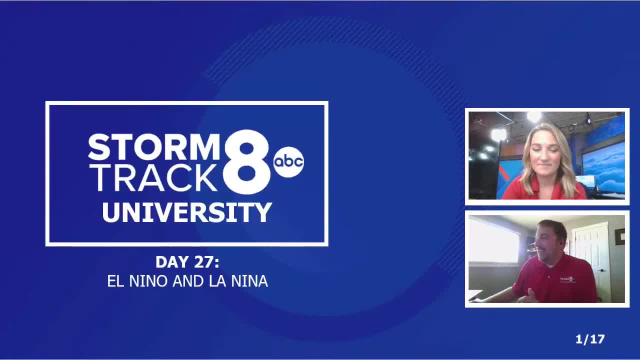 so that's, that's what my background noise and this is uh. anyway, i'll let you go ahead and go ahead and start a soft work, okay, yeah, so we're kind of in a continuation of last lesson. i think was just about two weeks ago. we went into long range forecasting, which we take a deep look at. 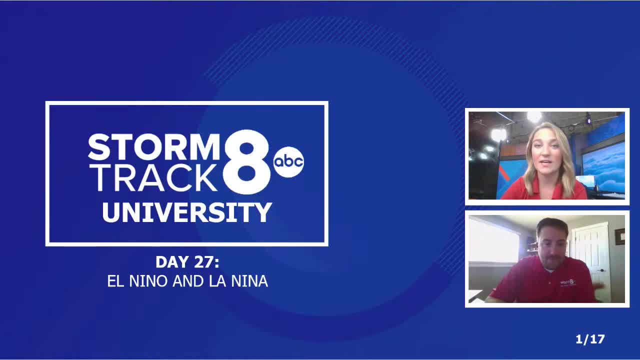 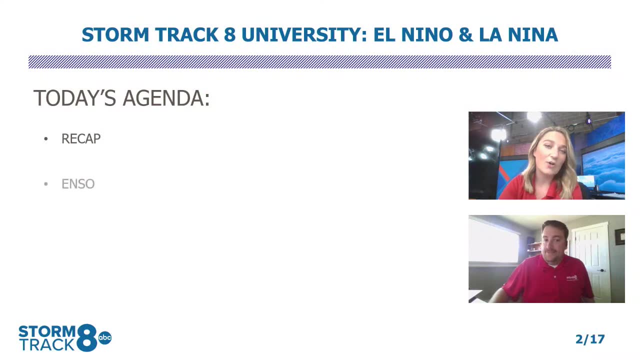 all these very large scale weather patterns that can stabilize for weeks, months, even years, and the most common one that we talk about and that almost everyone knows has heard of it, that would be the enzo teleconnection, which is where we get the el nino and the la nina patterns to take place. so 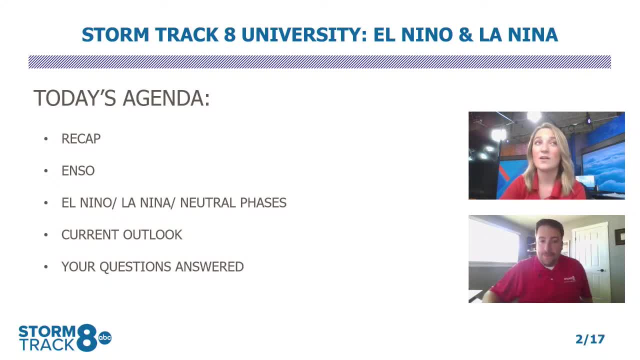 we're really going to do a little bit of that, and then we're going to do a little bit of the dive into this, because it can really influence our weather patterns and the different types of seasons that we get, whether they're more mild, whether they are more wet, whether they are more. 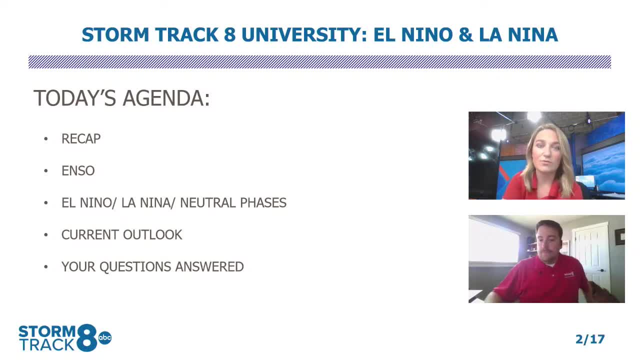 active. all that stuff can be correlated to whether we are in an el nino or a la nina. so on the agenda today we'll recap a little bit about kind of that long range forecasting, dive into the enzo teleconnection, break down the different phases, which would be el nino, la nina and the. 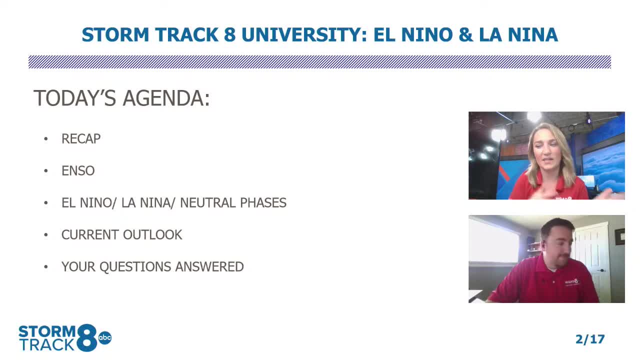 long range forecasting, then, of course, the neutral phase. then we'll take a look at where we are heading to right now, because we actually just recently saw a phase change, so we'll go into that. yes, how relevant and how timely this is that it matched up with that announcement. 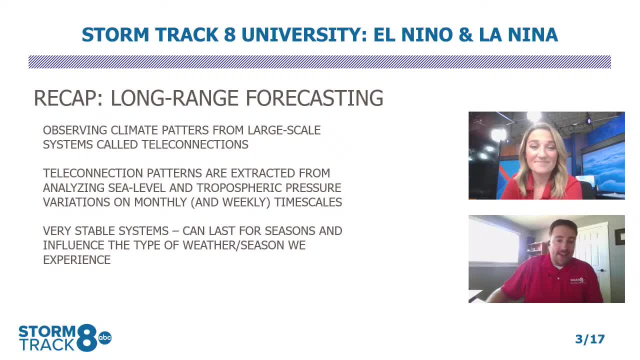 coming out literally, i think, just days ago, uh, from when i read that. so that's, that's something exciting and relevant that we'll be talking about today too. uh, so, to give a brief recap on what we talked about last time, we talked about long range forecasting. fine, take that paper. 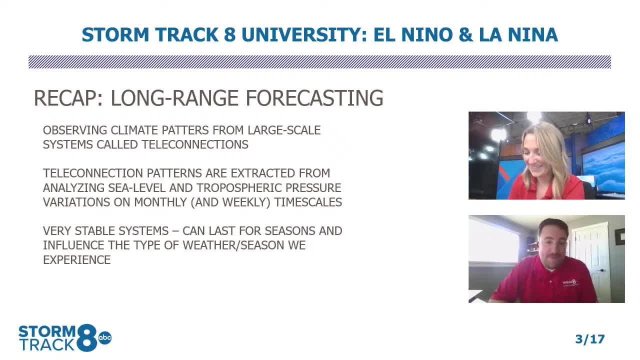 so we talk about long range forecasting. we're talking about observing climate patterns from large scale systems called teleconnections, and those teleconnection patterns they are extracted from analyzing sea level and tropospheric pressure variations on a monthly and weekly time scale. so we're not talking about hourly, daily, like we would with kind of our short-term forecasting. 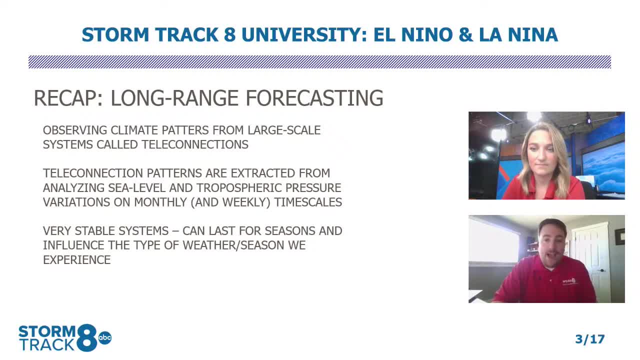 people. this is a much longer time span, a lot more complicated. we're talking about very stable systems that can last for seasons, and they can also influence the type of weather and season that we experience, hence the one we're talking about today. we're talking about today. 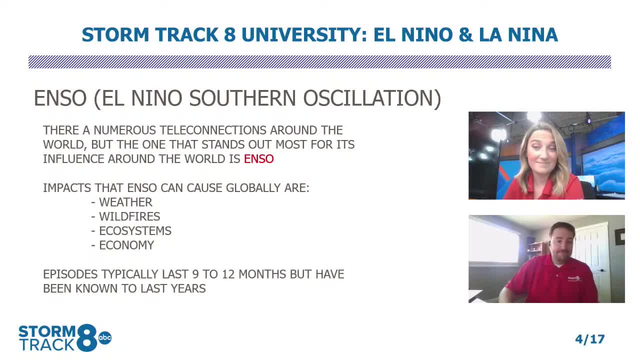 which are el nino and la nina. now enzo stands for el nino, southern oscillation. there are numerous teleconnections around the world, but again, the one that stands out most for its influence globally is, and so this is a very strong, large and stable teleconnection. the impacts: 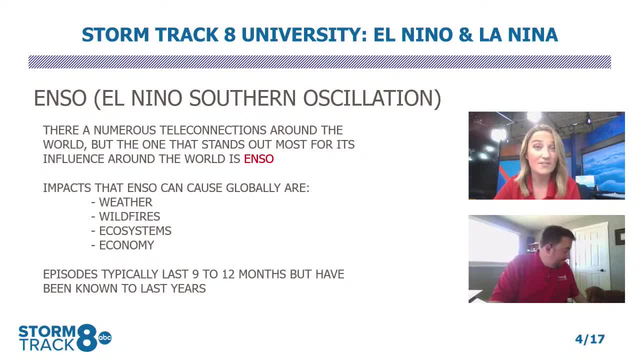 can cause globally are weather, wildfires, ecosystems and even can have some economic impacts on us, these episodes, or we're in again a neutral phase, we're in a la nina, we're in el nino, all that stuff. those episodes typically last around 9 to 12 months, but we've also seen these things stabilize. 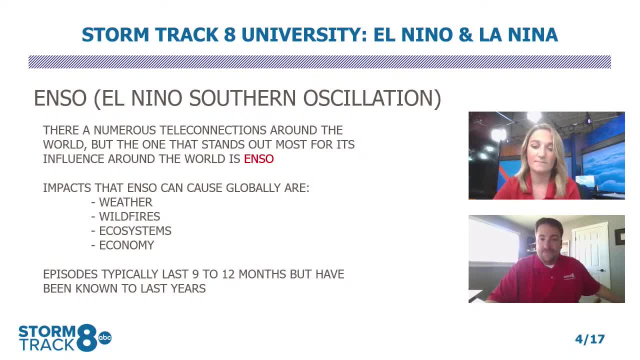 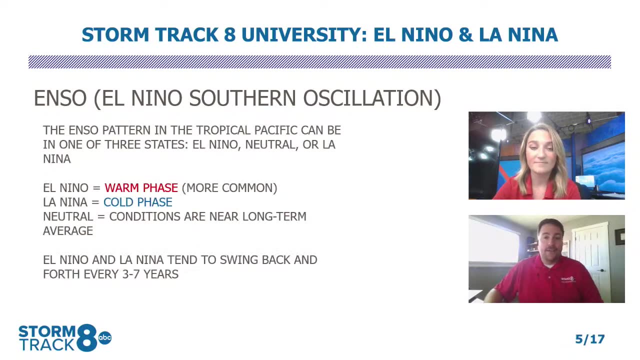 for years at a time. yeah, and that's a big list of what enzo can actually cause every season, and it's not just weather, it's just, it's not limited to any, uh, a certain category, if you will, really is far-reaching, uh and very broad. so the end zone, when you're talking about el nino in 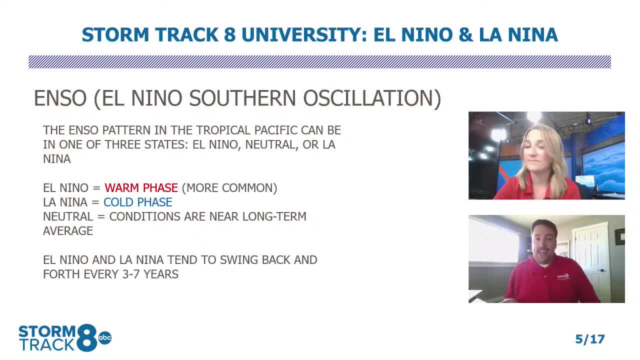 the southern oscillation. that's, of course, in the tropical pacific and it can be in one of the three states. it can be an el nino state, a neutral state or a la nina state. la nina state is the one that we just got out of. uh, it was with us for much of last fall and all of this winter, of course. 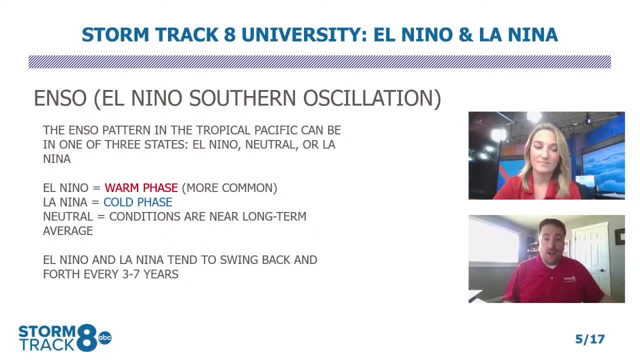 so when you're looking at el nino, you're looking at a warm phase which is more common. la nina is talking about the less common cold phase and when we're talking about these phases, we're talking about the uh service of the water. the water temperature in these uh different. 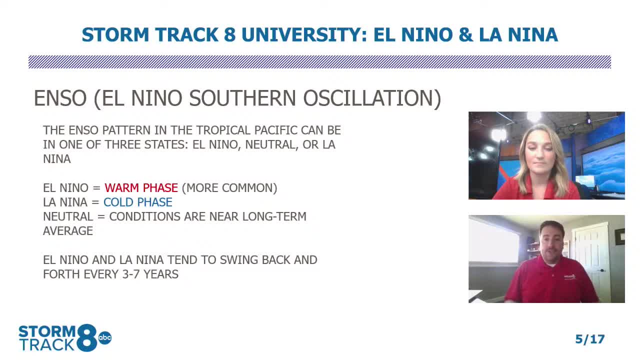 locations. when you're neutral, that means your conditions are near the long-term average. there's not a real big discrepancy there. el nino and la nina: they continue to swing back and forth every three to seven years, so it's almost like they're on a cycle with each other. you'll get one followed. 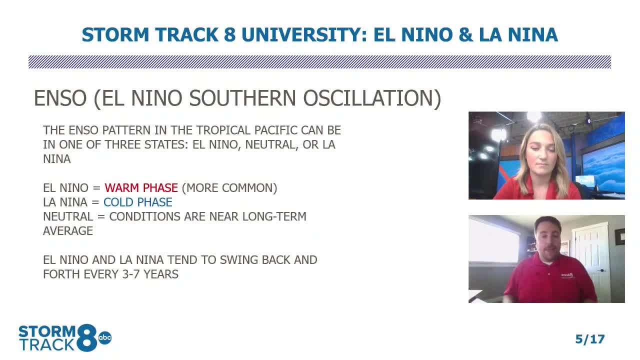 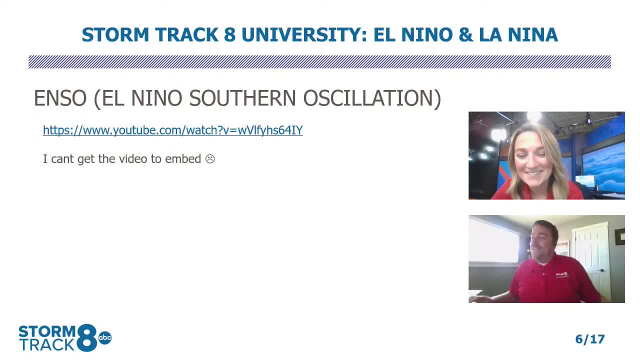 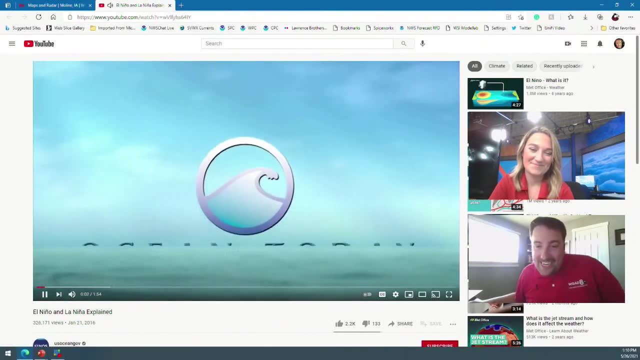 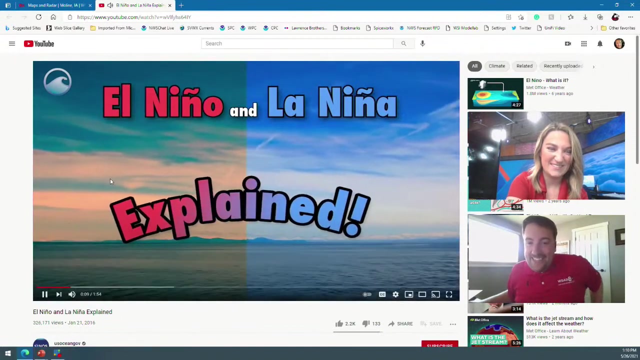 by a little bit of a neutral state control period and then sling back into the other. I couldn't get this to embed. I forgot to take it out. That's okay, We'll get it to play. That's funny. Warmer or colder than average ocean temperatures in one part of the world can influence weather. 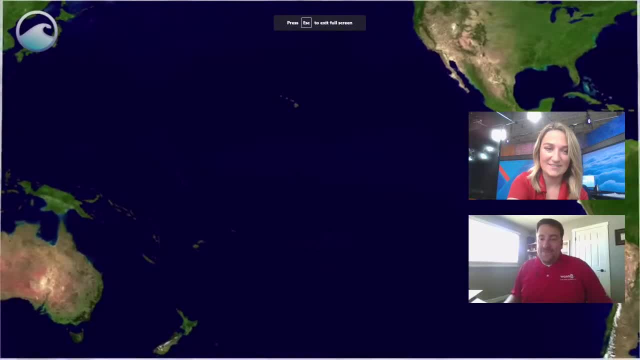 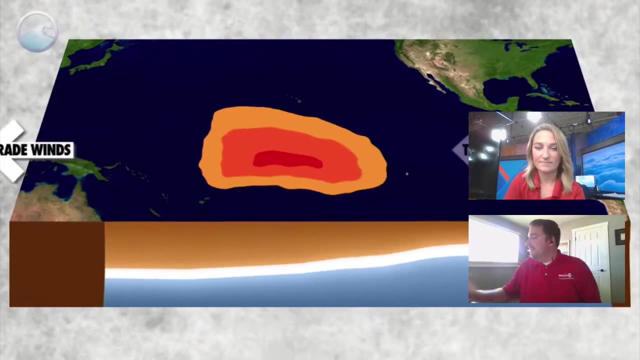 around the globe Boggles the mind right. Here's how it works During normal conditions. trade winds, which blow from east to west, push warm surface waters towards Asia, piling it up in the western Pacific. In some years, though, the trade winds weaken. 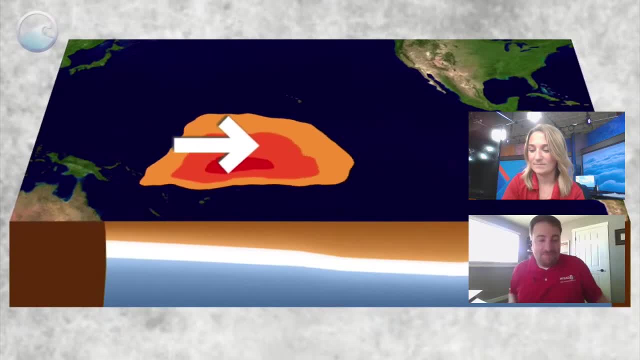 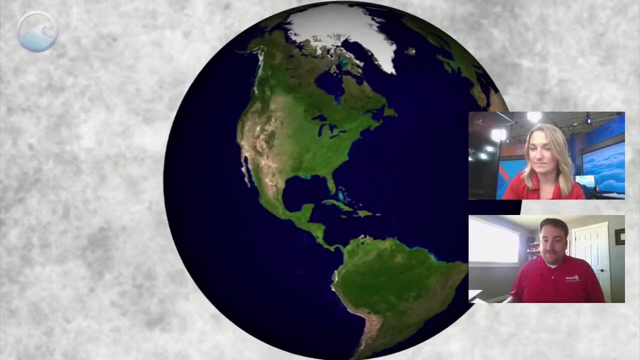 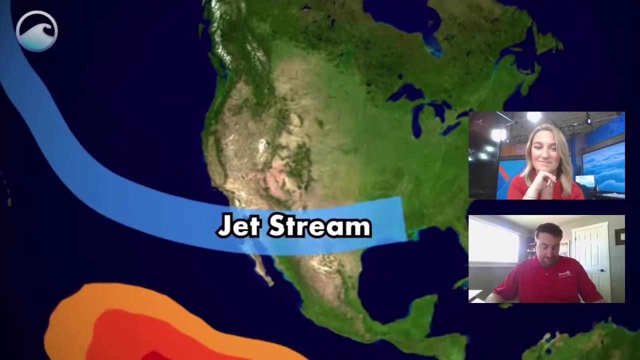 The warm surface water moves eastward and reduces upwelling of cold water off the coast of South America. Climatologists call this El Niño. Its climate impacts show up mostly in the wintertime. over North America, The warmer ocean fuels an intensification and southward shift of the jet stream. 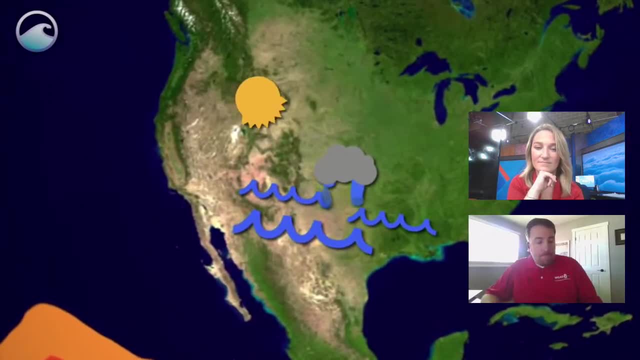 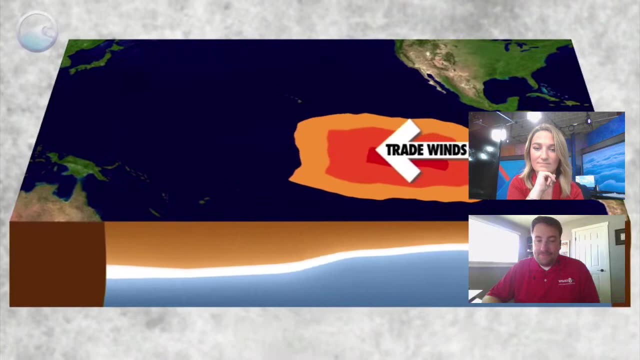 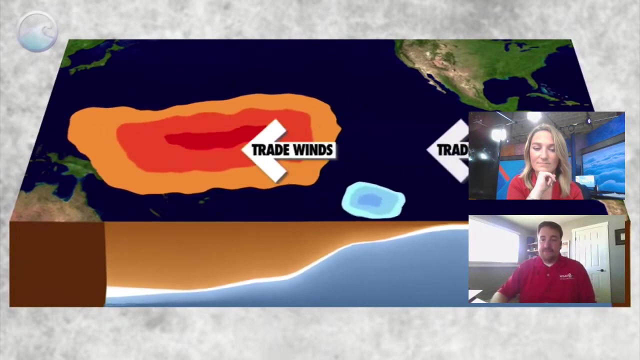 This brings flooding to the southern United States and warmer, drier conditions over parts of the Pacific Northwest, northern US and Canada. But eventually those trade winds pick up again and sometimes become even stronger than normal. When that happens, they blow the warm water back into the western Pacific and restart. 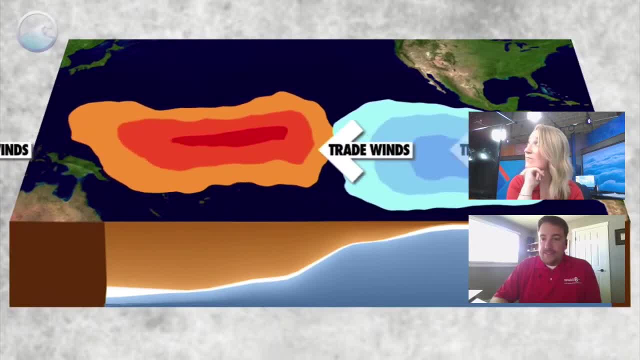 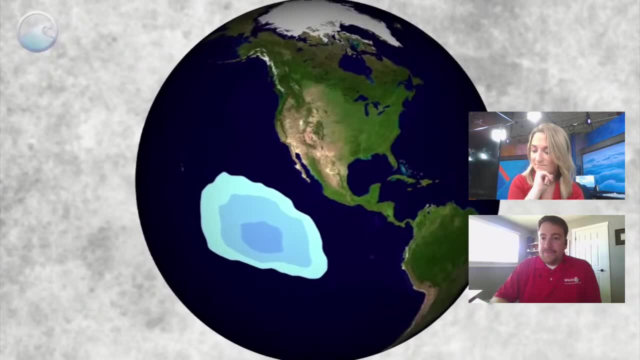 the upwelling of cool water towards the surface in the eastern Pacific. These strong trade winds are a signature of what is called La Niña: Unusually cold, Unusually cold conditions in the tropical Pacific that displace the jet stream northward. 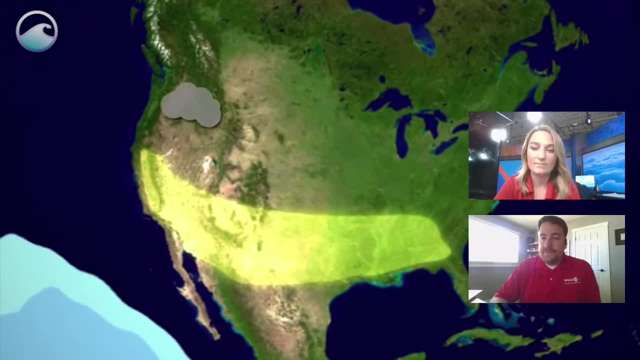 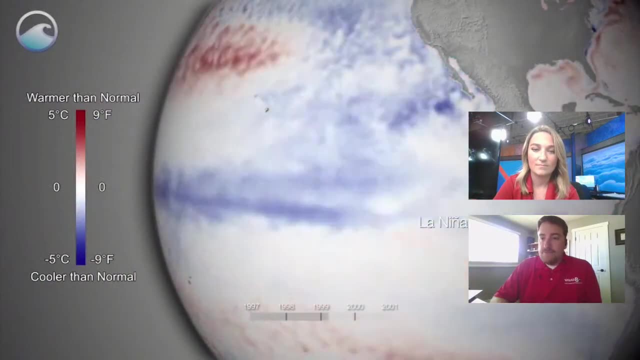 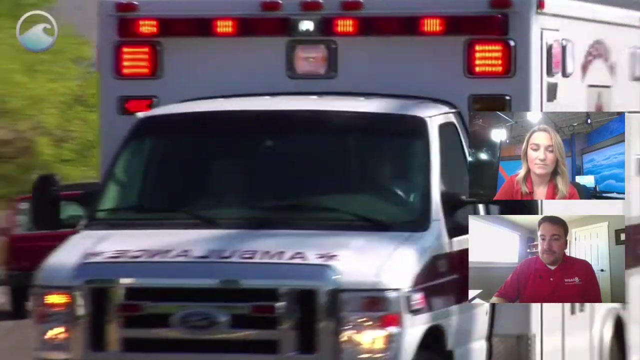 La Niña can lead to drought in the southern US and cooler temperatures, heavy rains and flooding in the Pacific Northwest. El Niño and La Niña together are part of a cycle that influences extreme weather and can impact food production, water supply and even human health, not just in the US. 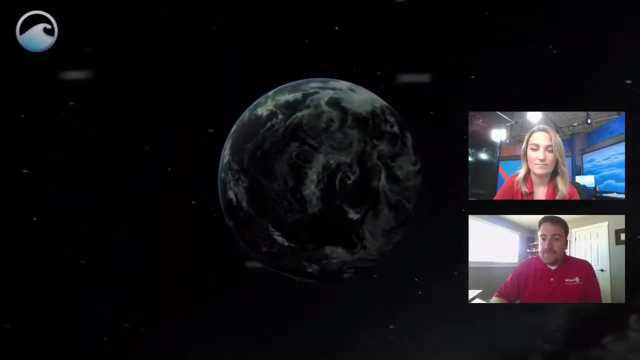 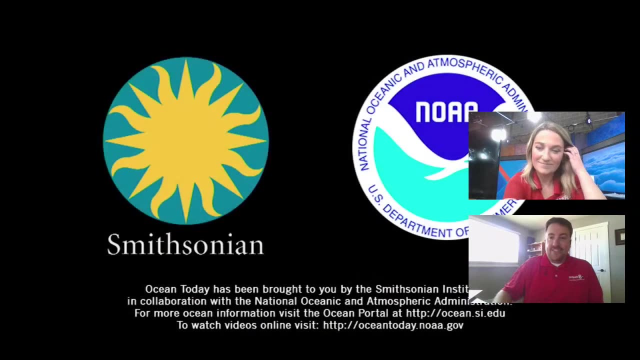 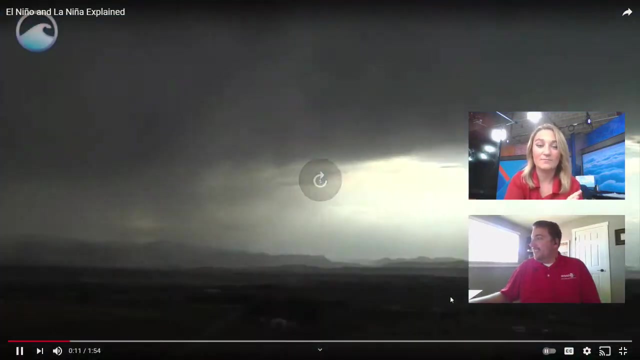 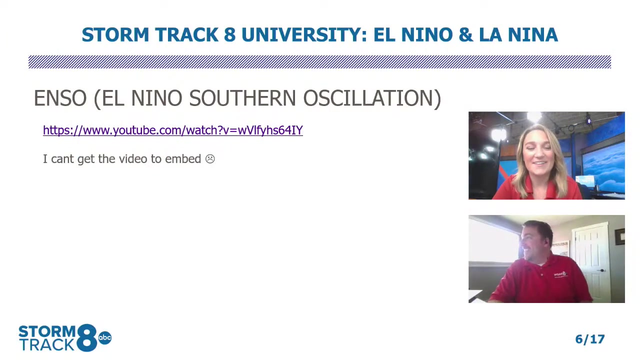 but in many parts of the globe Good stuff. Yeah, that was just a little bit of an overview about El Niño and La Niña and how weather or normal condition and how the impacts are caused by the sea surface temperatures and weather. 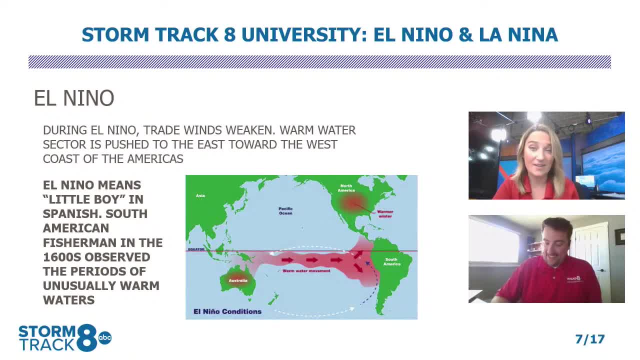 We are warmer, specifically on the Americas, Off the coast of the Americas, Okay, Like we are in El Niño. So diving into that during the El Niño again, those trade winds which we do find. this is talking about upper levels. 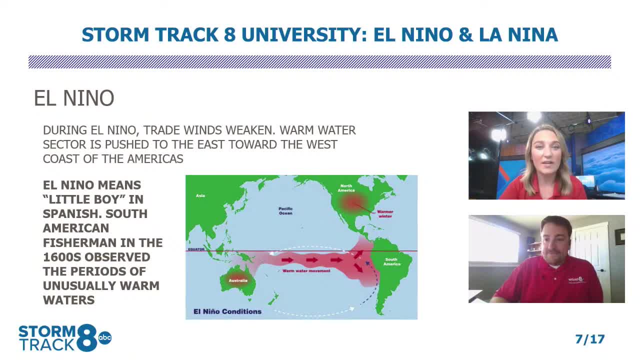 So not really anything that has to do with that surface, but these trade winds will weaken, And when those trade winds weaken we get that movement of the warmer sector of water to really shove itself over on the western coast of the Americas. Again, this is something that happens more commonly. 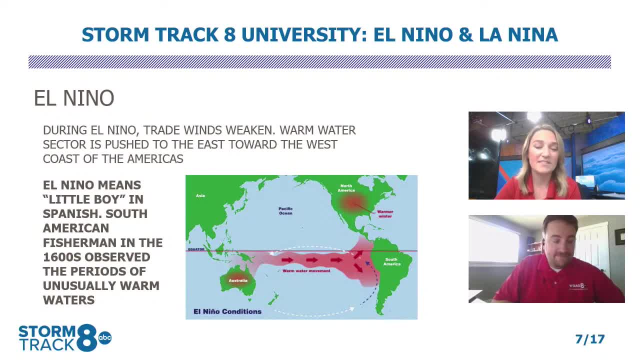 Although we were just in La Niña. but El Niño in Spanish means the little boy, And again, this kind of was discovered in those areas as well. So it's very obvious as to why we call it El Niño. but South American fishermen actually. 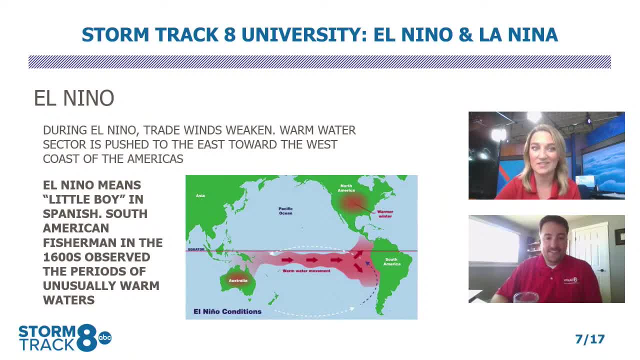 were the ones to observe this pattern change in the 1600s. They were the ones that observed how we were getting unusually warm waters in different periods. So So it does show that a lot of people are observing. again, we talked about how our farmers out. 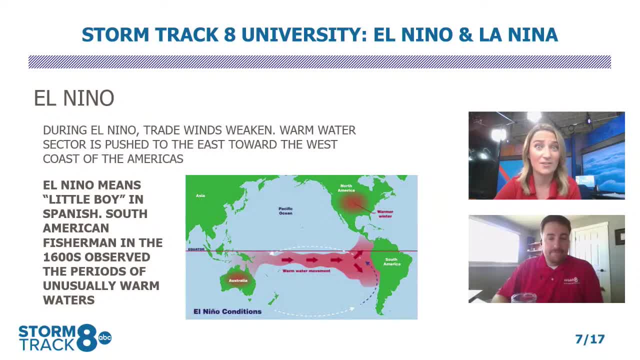 here in the agriculture industry so well-knowledged on the weather, because they're constantly observing this, Yeah, And you think about a lot of our farmers around here who have been doing this for generations upon generations and they've been able to see and witness firsthand kind of these long. 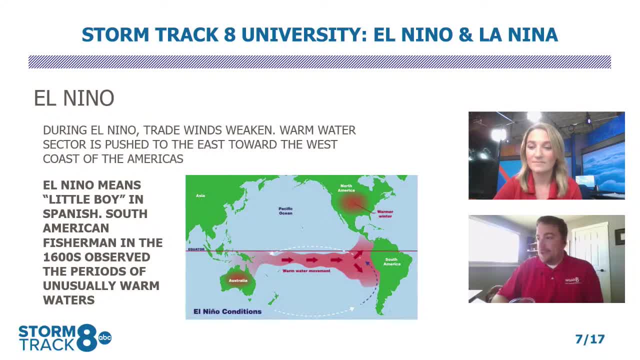 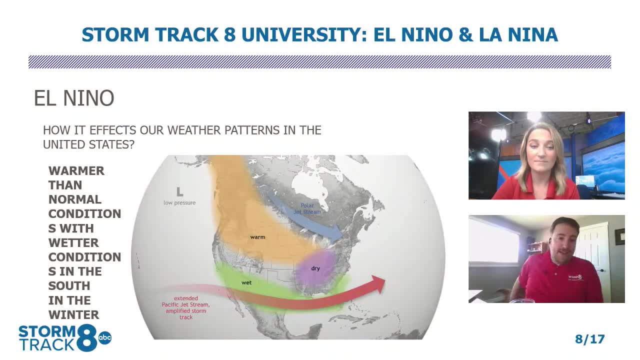 term effects of these two phenomenon, which also drives a lot of credit and credence, if you will, to just how powerful these things are. Let's look at El Niño again and see how it affects our weather pattern in the United States. 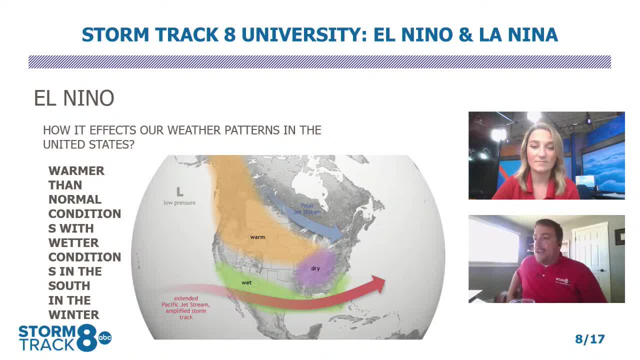 So here it has a couple of different impacts. So if we look at the map there in the center of your screen, you notice we're kind of on the edge of that drier pattern and also on the edge of the warmer pattern too. 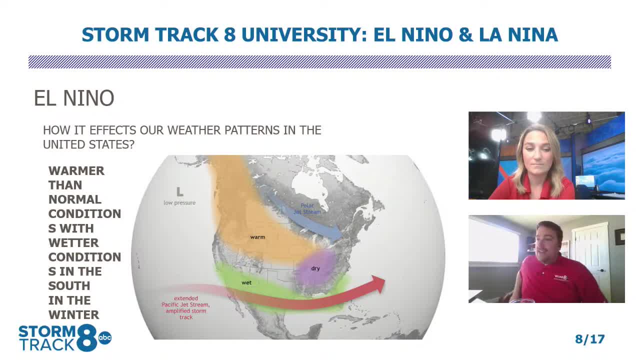 But generally speaking, when you have an El Niño, that's something that I'm usually a big fan of around here, and a lot of folks that don't like winter are a big fan of it, because we usually typically are warmer, It's a mild, easy winter for us. 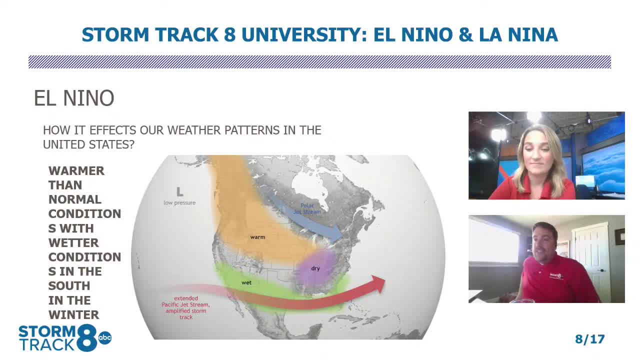 We have warmer than normal conditions, wetter conditions in the south in the winter. You'll notice too during El Niño that the Gulf Coast really gets a lot of the storm systems that develop as you go through not only the winter but the spring as well. 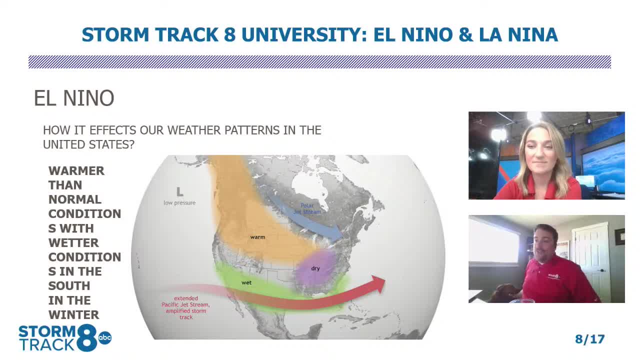 That jet stream, the extended Pacific jet stream and the amplified storm track are well to the south. But look at the polar jet where it is well to the north, So that keeps all that nasty polar Arctic outcast. That's a great area, if you will, well removed from us. 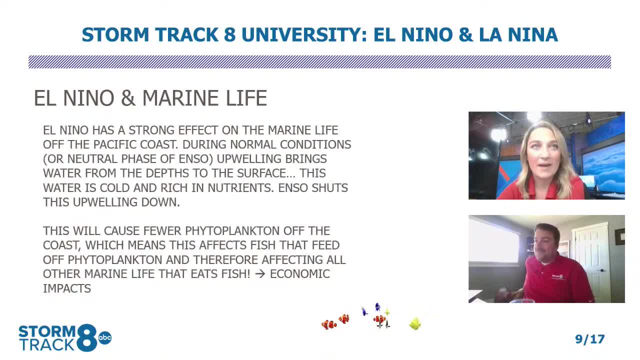 Yeah, Absolutely. I think El Niño would be a pattern that the south would love to be in right now because they are struggling, especially on the southwest, with those drought conditions. Unfortunately, we haven't seen an El Niño for a little bit. 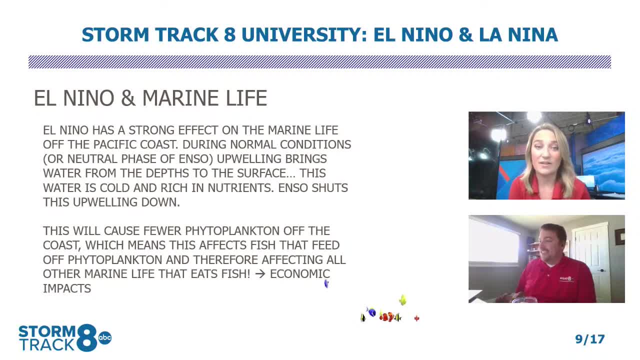 So El Niño can have an impact on marine life. El Niño has strong effects on the marine life, specifically off that Pacific coast. It's just like the other ocean. It's a little bit more of a coral, It's a little bit more of a Pacific coast. 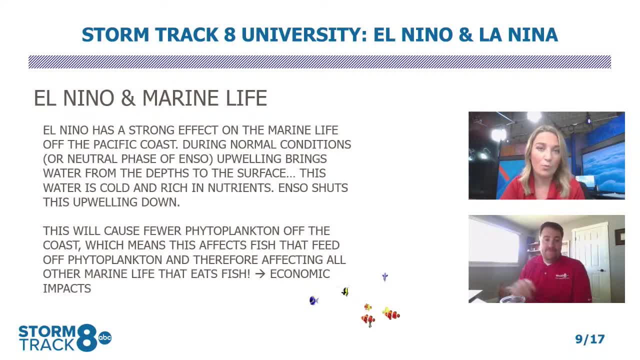 But it's also a really strong and strong ocean. We've seen it for a long time but we don't see it here. But when Enso is in that El Niño phase or that warm phase, it's kind of shutting down. 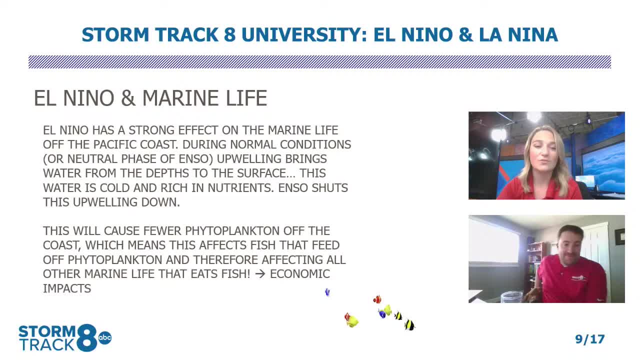 that upwelling So we're not really seeing that cold, nutrient-dense water come back up to the surface, which really helps marine life. so this will cause fewer phytoplankton off the coast, which means that affects the fish that eat the phytoplankton and therefore affecting all other marine life that eats those fish. so we 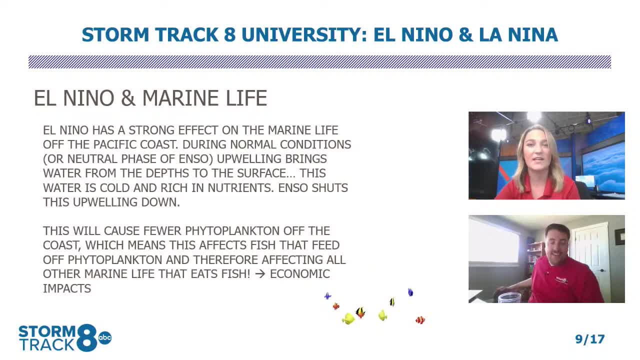 do see actually economic impacts from that. when it comes to fishing season and we're in an El Nino pattern, yeah, really it's like dominoes: you get one thing to what to change and it just constantly changes the other things that interact as well. are we going to sit down for a second? uh, looking. 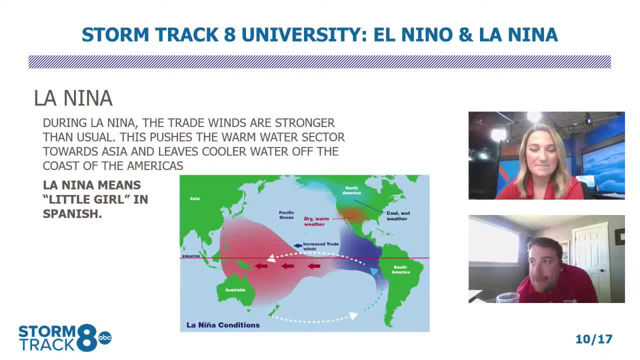 at La Nina, so you're looking at the complete opposite of this. so now you're talking about the trade winds being stronger than usual. so what this is doing is essentially pushing that warmer water away from the coast of South America and Central America, so you're getting a cooling effect. 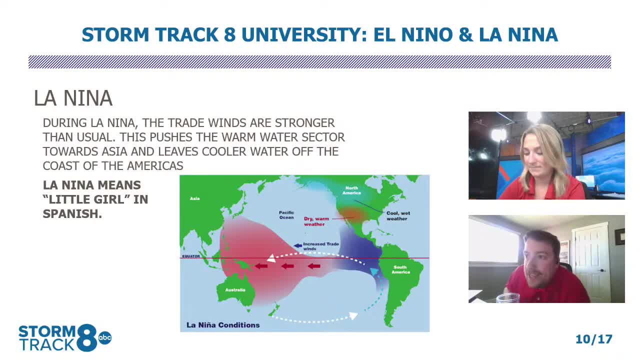 on the water and that what that does is it actually, of course, cools the water temperatures down, but you're also looking at big impacts to the weather pattern here in North America, for example. look at the map here. we're going to amplify this on the next slide. as you can see, there's a lot of dry weather in the Southwest. 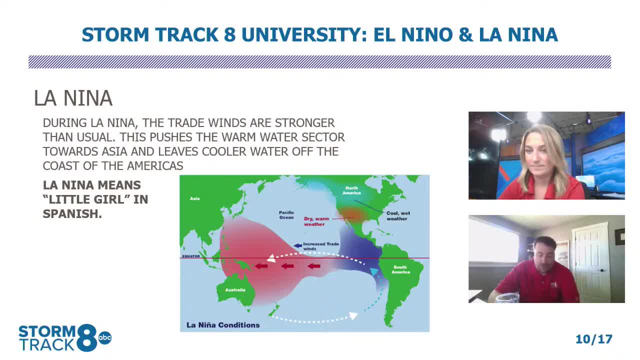 think of what's going on right now in terms of the drought situation across portions of California and Arizona. it's pretty dire right now and that matches up really well with the fact that we just went through a La Nina and if you look at the- the meaning of the word, it means a little girl in. 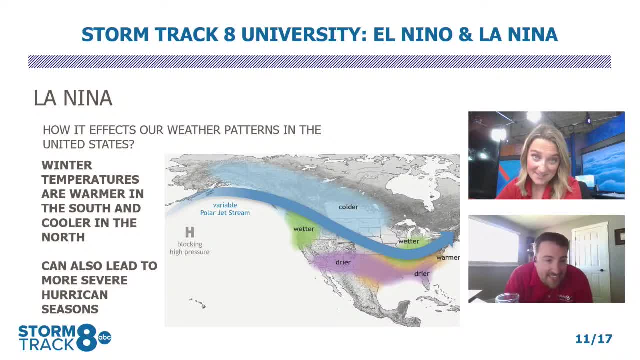 and now affects us, where it's pretty much again matching up to what we just experienced with this past winter. uh, winter temperatures are warmer in the South and, of course, drier, so they are still stuck in that drought, and it did did become a lot more severe over the winter because they were not getting 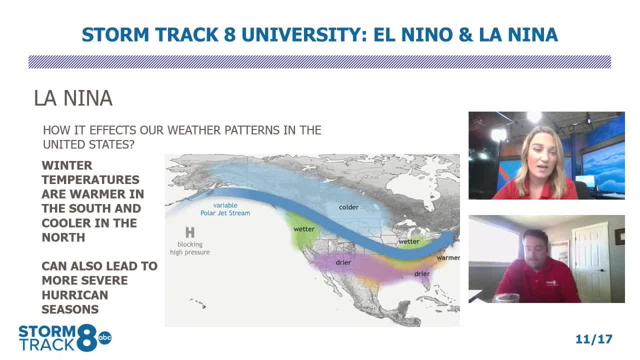 that they didn't really get their monsoon season that they experience, and then cooler in the north, which we all remember, February. we were just locked underneath that polar air for what seems like days on end in February. This can also lead to more severe hurricane seasons, which is something that we also just experienced. 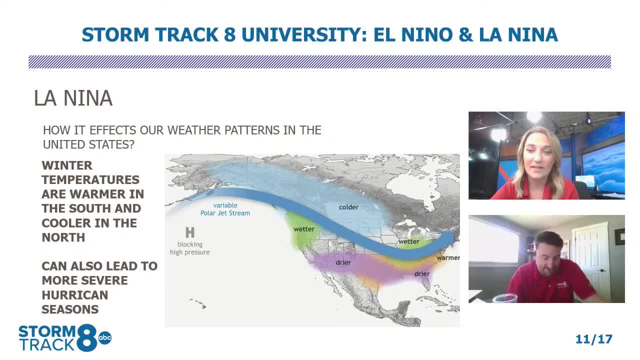 But La Nina also is known for kind of amplifying storm tracks. here in the United States as well. We were kind of looking forward to our severe weather season because we were expecting or hoping that La Nina would hold on for a little bit longer. but of course it. 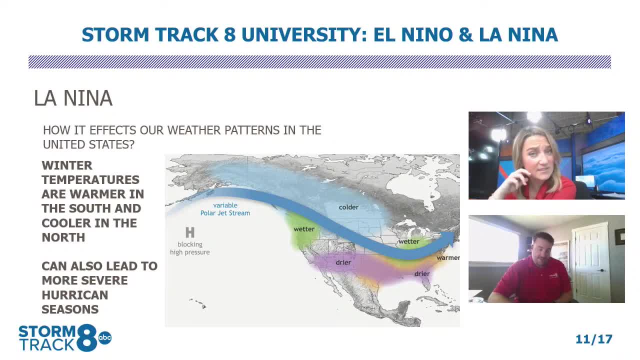 has shifted since, But definitely the south near the Gulf Alabama has been getting hammered so far with severe weather which could have been a little bit more of an influence from La Nina in the past couple of months. Yeah, definitely, You've seen that uptick. 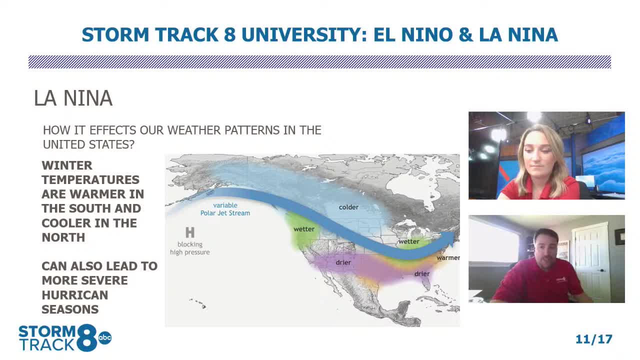 in correlation to what's going on with La Nina. And now that we're in neutral, you were kind of thinking, well, maybe it would go a little bit further north with time, but we just haven't seen that yet. So there may be some filtering effects. 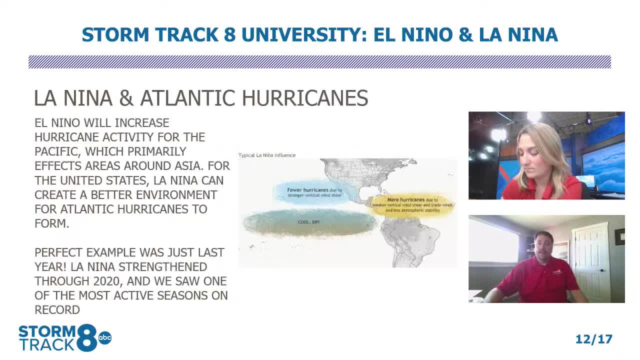 with that, but we'll see if that kind of straightens itself out here in the next several weeks. If you look at the connection to La Nina and some Atlantic hurricane activity, so La Nina will typically increase the hurricane activity for the Pacific Ocean, which makes sense because you're 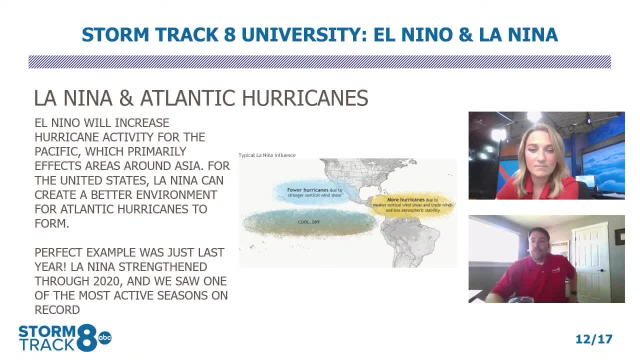 talking about warmer water there, So that primarily affects areas around Asia, The United States, La Nina can create a better environment or, excuse me, the cooler. I got the interview. so, La Nina, you're doing with the cooler water, not the warmer water. that's La Nina. 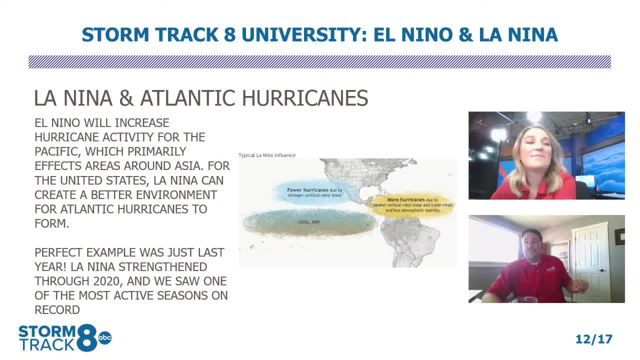 Strike that off the record, La Nina. it can create a better environment for Atlantic hurricane to form, and that makes sense because you're dealing with the other side of the continent there, not the western side. So a good example of this was last year, where we had La Nina that strengthened. 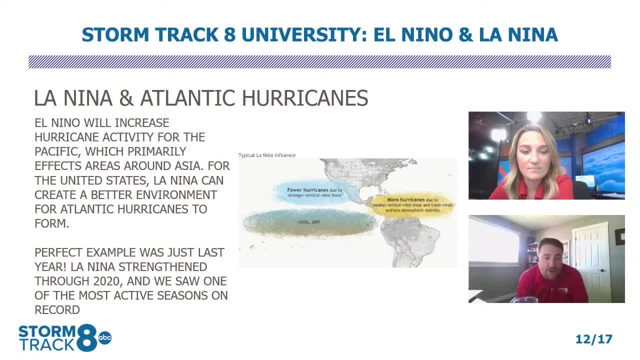 throughout 2020.. And we saw one of the most active hurricane seasons on record. Do you remember that, where we went clear into the Greek alphabet And it seemed like it was never going to end? and it eventually did, of course, but it was a very active year. 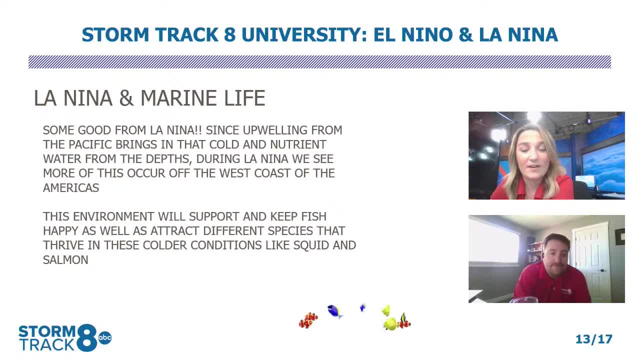 Absolutely, and 2020 is to blame, actually, for the Greek alphabet being officially retired now for hurricanes. Now we have a supplemental list that will use names, because they do want to retire a couple of those Greek names because they were too disastrous, So they had to go with a. 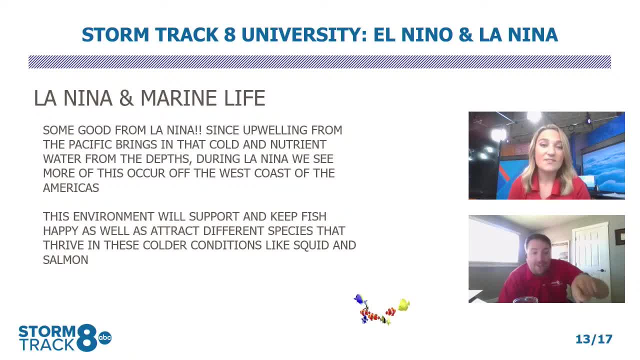 different route, which is crazy Plus side for us that work in the TV business. they were hard to say, The names were hard to say, They were so hard to say. All right, so we have something that's good. It just sounds like La Nina. 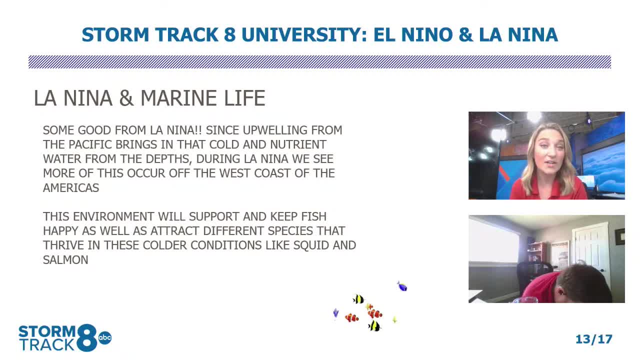 causes a little bit more problems for us, but something that is good when it comes to La Nina is the impact that it does have on marine life Now, since upwelling from the Pacific brings in that cold and nutrient-dense water, well, upwelling is amplified with that colder water. 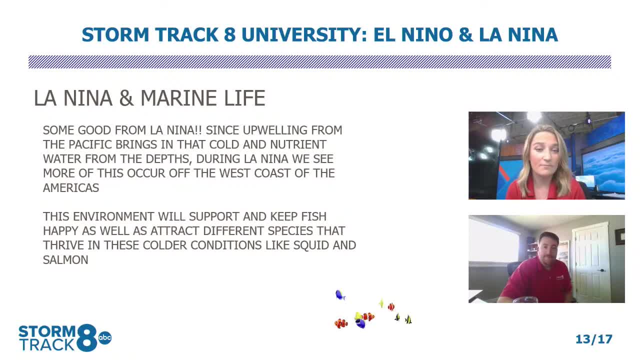 during the La Nina, especially off the west coast of the Americas. So this environment will support and keep those fish happy, as well as attract different species that thrive in those colder conditions, like squid and salmon, And nobody likes a sad fish, We like happy fish. 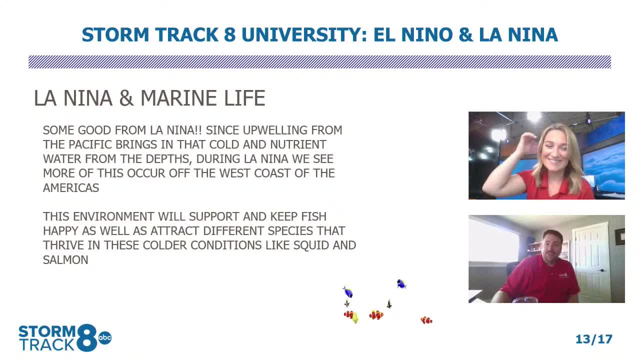 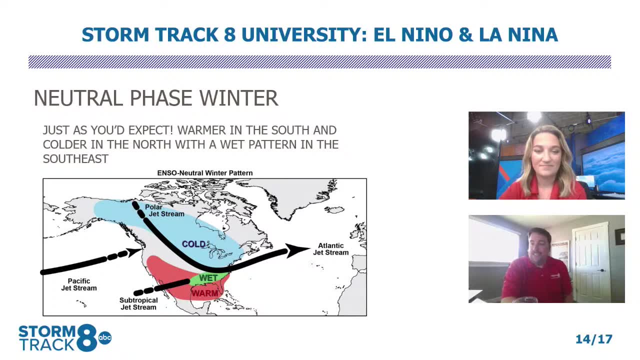 No one likes a sad fish And that certainly makes them happy. If you look at the neutral phase of winter, notice on the map that our Atlantic jet stream and attached to the polar jet stream of course it's a lot closer to us. So, yeah, we get those. 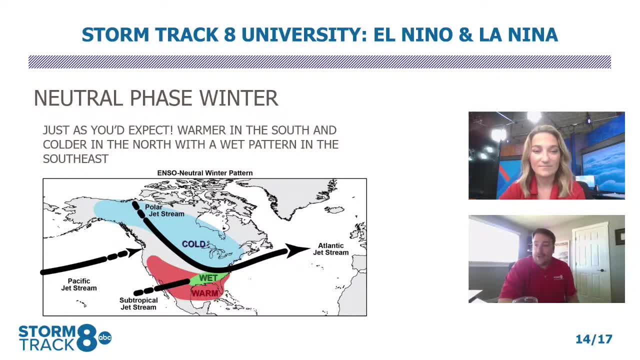 occasional cold spells, Also wetter and warmer to the south and east. That's why Florida is such a popular destination, of course, during any winter month, it seems. But just as you'd expect, of course, warmer in the south, colder in the north, with a wet pattern in the southeast. all tied to 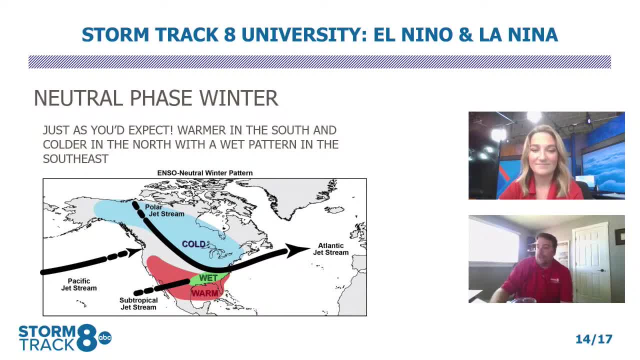 that jet stream and where it's located in relation to the colder and the wetter. So if you look at that, it's a lot closer to us than it is in the south, So it's a lot closer to us than it is in the. 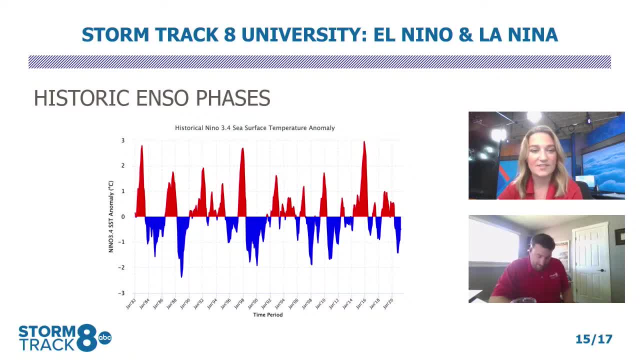 north, So we're going to have a lot more bear passes. There's a look Once again. we touched on this with our last lesson, but, just as the historic ENSO phases, this is looking all the way back from 1982 to 2020.. And it does go back and forth. 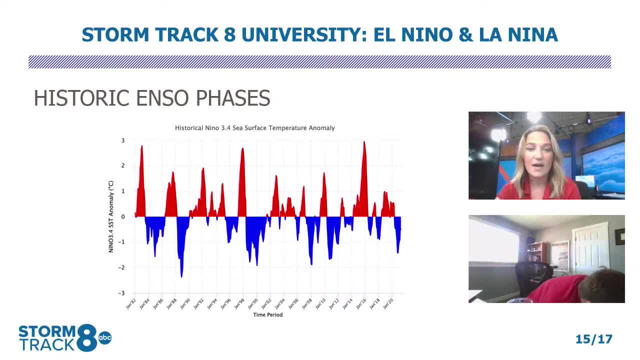 some severe, some closer to that neutral phase, But you also can kind of notice that there is a little bit more peaks on that El Nino side or that red side, So kind of proving that it's more common, but also something that we're going to be able to see in the future. So we're going to 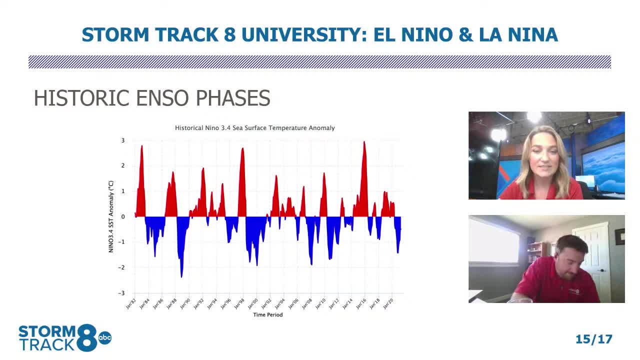 be able to see that. So we're going to be able to see that. So we're going to be able to see that. interesting that I am observing that it kind of looks like La Nina can kind of hold on for a little bit longer. instead of it just looks like El Nino has those short, quick peaks and then La 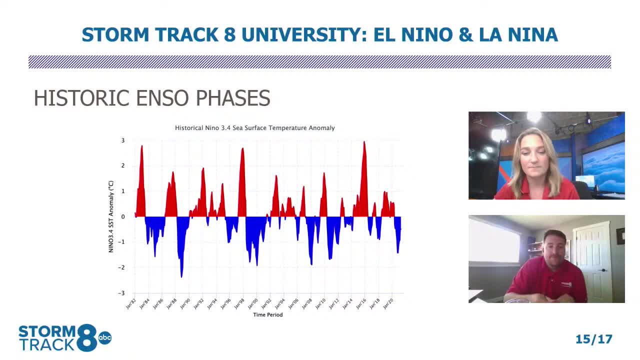 Nina has a little bit longer duration periods. Oh, you're muted. Okay, There we go. Now can you hear me? Yes, Don't pull the cord out. That's not very nice. So, yeah, the graph. yeah, we talked about this last time too, and that you notice that. 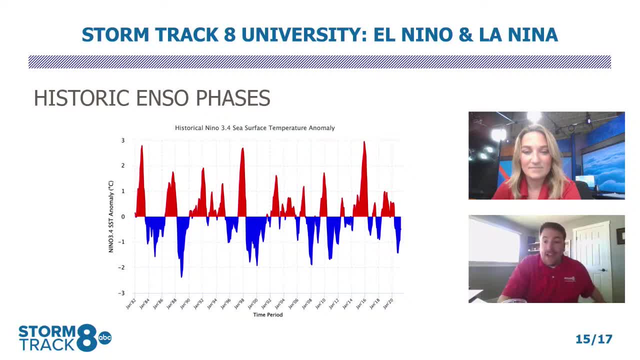 if you look at the warmer phases, they're more pronounced, They have a lot more weight to them than the colder phases do, And you'll notice that too if you look at past La Nina events, per se or El Nino events. if you look at the magnitude or the coverage or strength of the warm 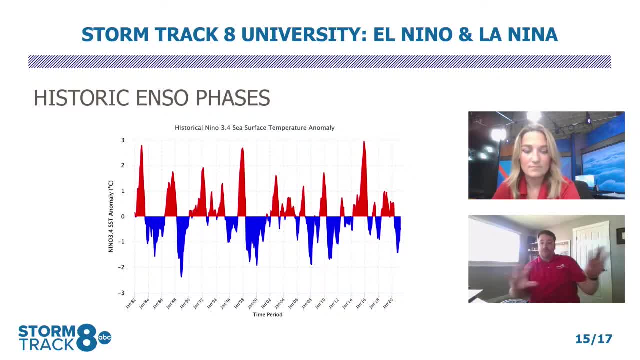 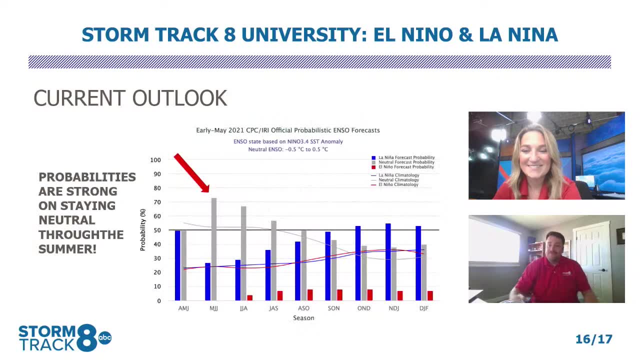 versus cool water that typically El Nino is going to have more far-reaching effects in terms of the distance. It's going to have more water compared to La Nina. All right, All right, One more slide. You can do this. Let's look at our current outlook, which, again, this is kind of going through the year ahead. 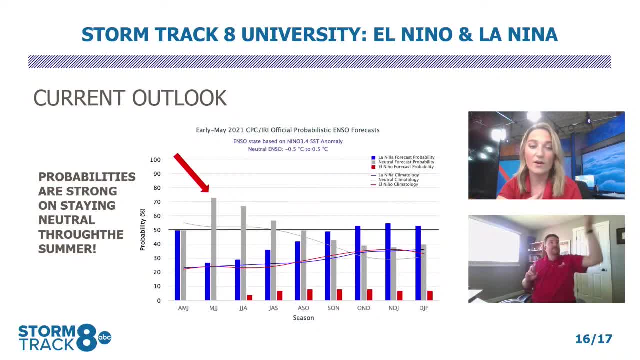 This was just updated, I think a couple weeks ago, But we are at that. I put an arrow where we are, where we're looking at May, June, July, which it does look like we are most likely going to be in a neutral phase going into. 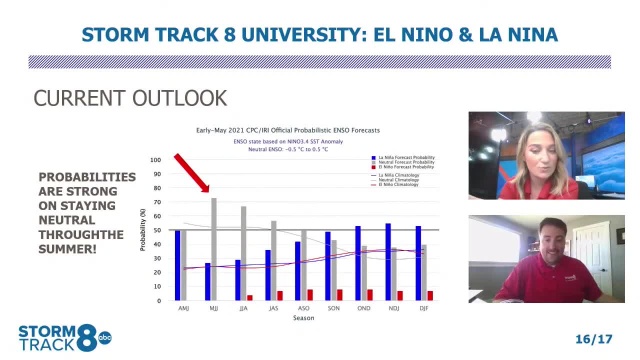 you know our summer seasons But if you pay attention to the end of that graph where we're kind of getting towards the winter months, maybe hinting that we could see a little bit more of a La Nina influence once again as we head into the winter. 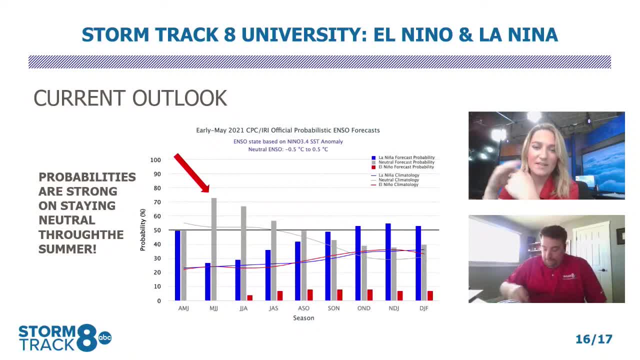 Of course, this is an outlook. This can absolutely change And you can also see the probability goes much goes down a lot as we go farther out. Again, this is an outlook, not a forecast, But it does look like, at least for the summer. 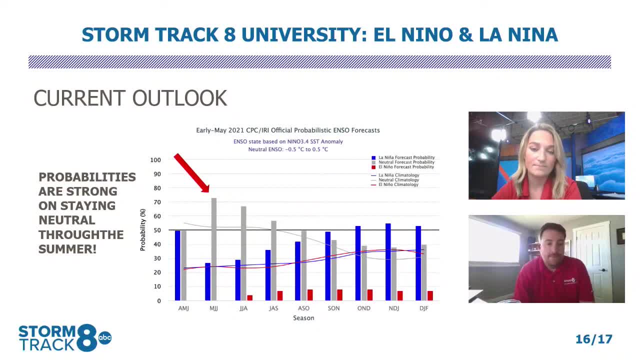 we are going to continue to see that neutral phase stick around. Yeah, that's what I was reading as well. It looks like it does favor that we will stick with the neutral phase, perhaps maybe getting into another La Nina by the end of fall, maybe next winter again. 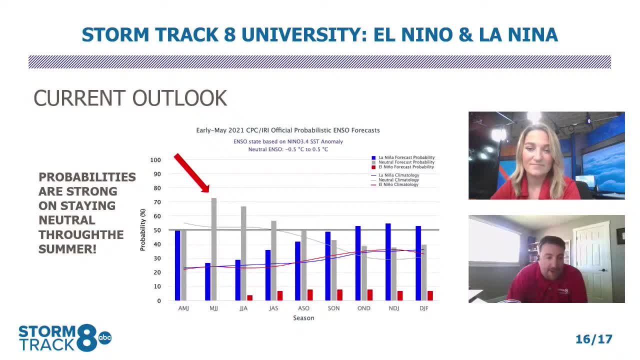 But it's really hard to predict these things so far in advance because again you're talking about a system you're not going to get with anyway. But it is nice that we're going to be going back into a neutral season, because what that does is it really helps. 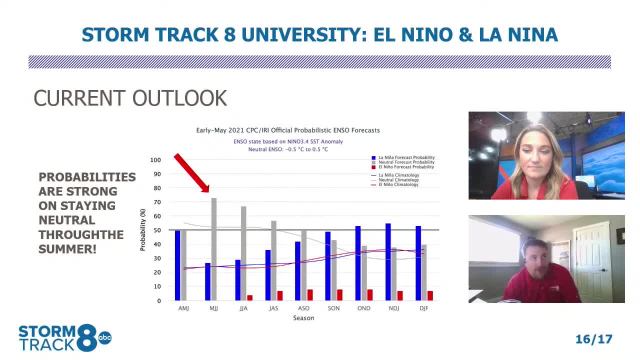 if you will improve the accuracy, if you will, of the long-range weather forecasts, because you're not having this obscure variable, whether it be La Nina or El Nino, playing a role in interrupting some of the normal patterns that we've come to know and recognize over the many hundreds of years that weather forecasting has been ongoing. 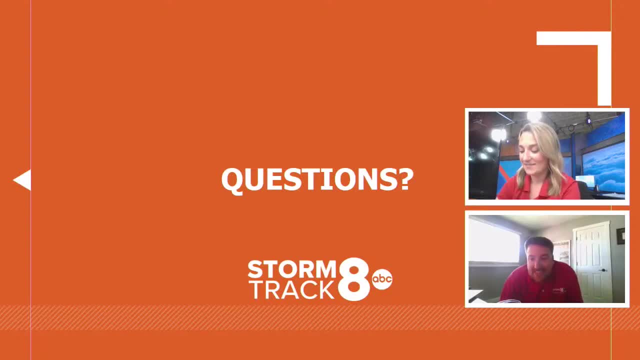 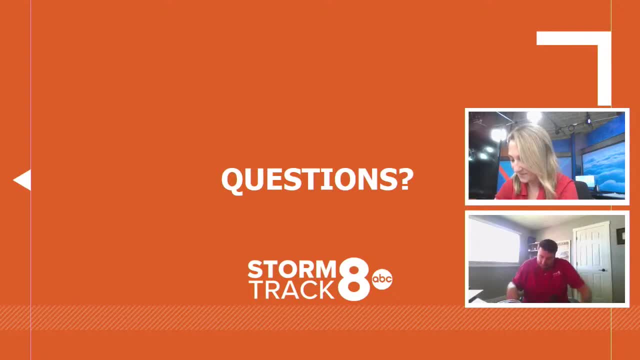 Hello Seth, Hey Seth, Seth checking in, And then I think I had a couple on my page. Where is it? Yeah, just a few Again, Seth checking in, And then Devin says what is the weather going to be for the next 10 days? 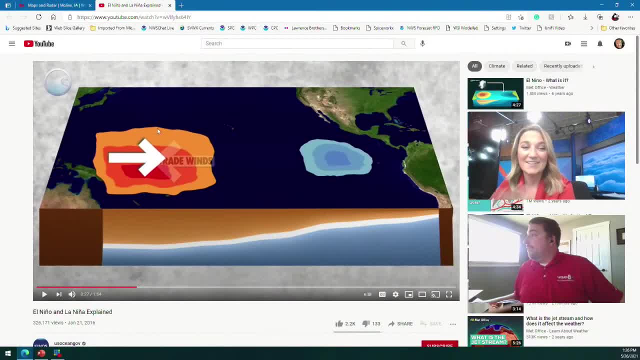 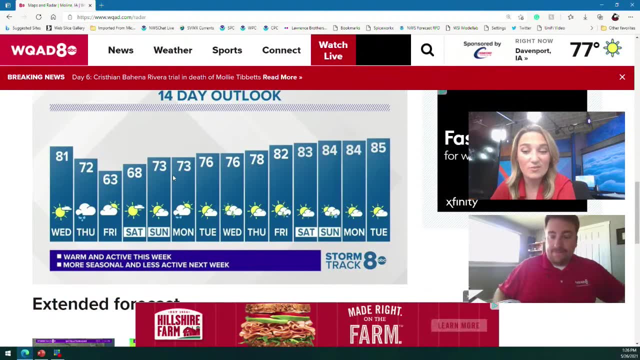 Whoa, Cooler, Definitely cooler, Cooler. I think Eric said it could be about a week, Yep, A week or so. Next 10 days we'll stay below that 80-degree mark, So we will be slightly cooler And then still seeing those chances of rain and some storms sprinkled in the mix. 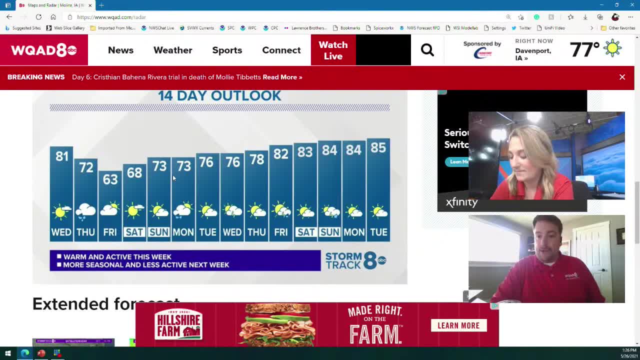 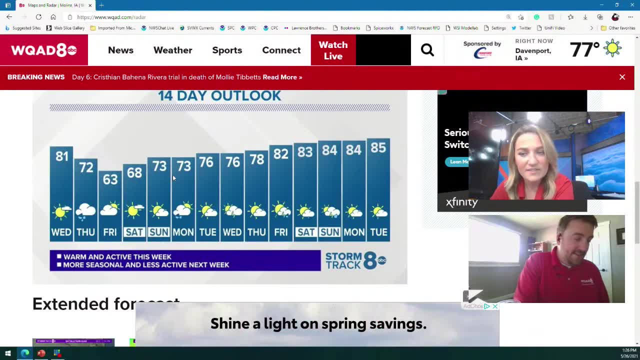 Yep, That looks about right, Which can't complain. I'm kind of excited to get my windows back open for just a little bit longer before we officially enter into June. Yeah, That will be nice to have that little period again. Give the electric bill a break. 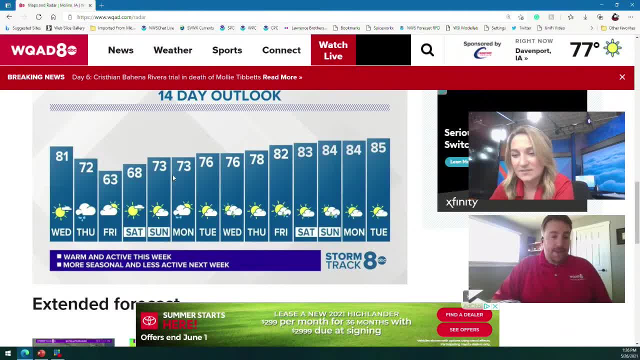 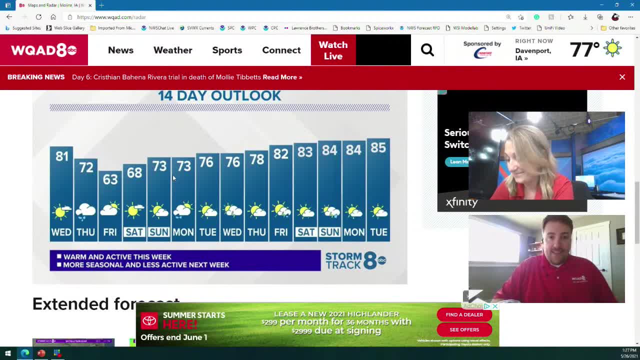 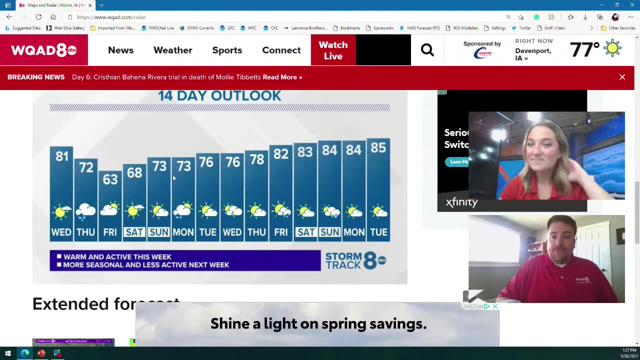 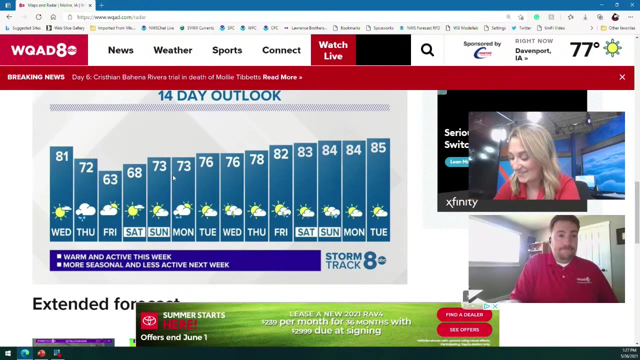 It's a great little thing, Mm-hmm. Now I'm loading up my page. Oh, there it is. Amy from Galesburg says: hello, Hi, Awesome, Is that it? That's all I got, All right. 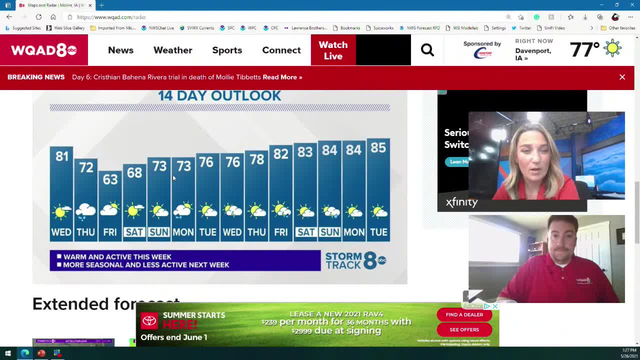 I think we have perhaps blocking patterns. I think you're right. I think that's the next one. Blocking patterns, That's another big one, And that may be our. that would probably be a good place to stop for our summer break too. 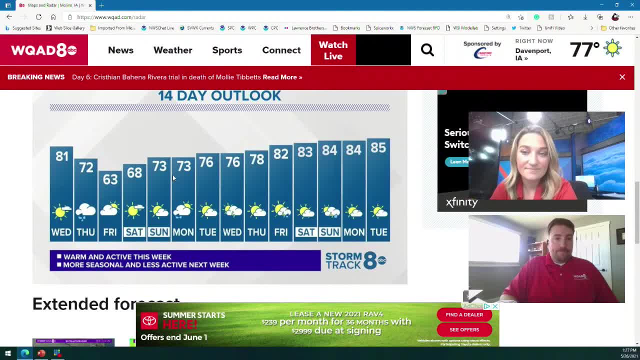 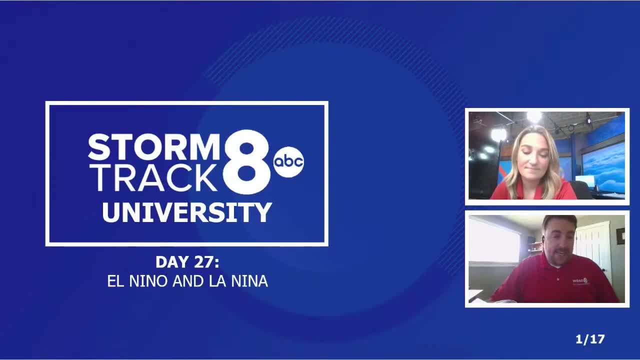 Cause it kind of ties in with what we did today a little bit before we try a brand new topic. So that will probably be the plan. We did take a little bit of a break last summer, cause we know schools are taking a bit of a break. 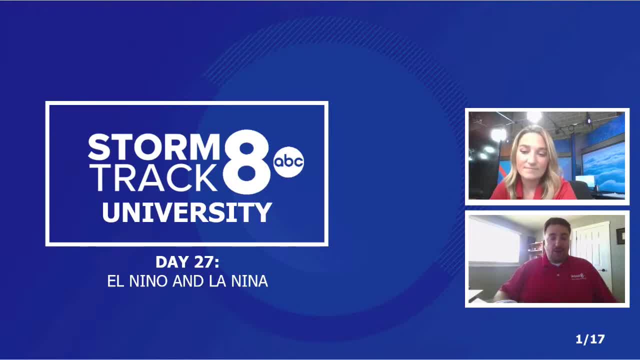 and you guys want to take a bit of a break too. We've got some other special projects that we're gonna be working on in the weeks ahead as well. They're gonna be on air online, all that good stuff. Yeah, I think that would be a good opportunity next week. 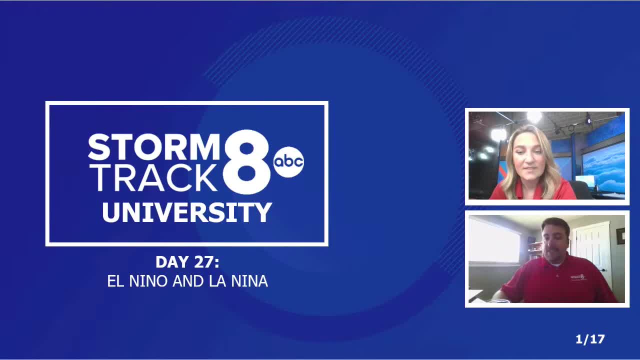 to have that be the season finale, if you will. Season finale, Except, don't expect a whole lot of drama. like you would on the batch, Like you would on the bachelor or bachelorette, Like nobody's gonna be crying, Nobody's gonna be jumping over a wall, or 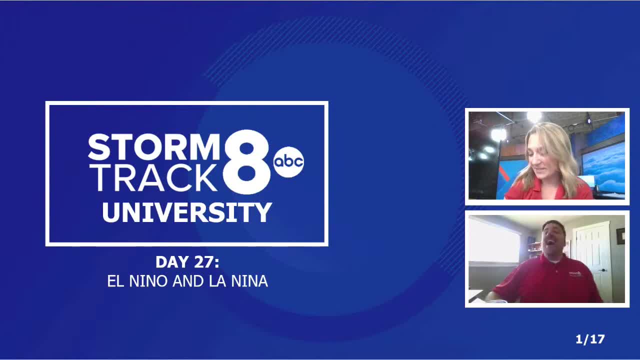 Don't expect any of that, Don't tempt me. That's true. Yeah, Morgan's back in the studio. I am. that's another exciting thing- All these tools and things that she could use that I don't have here at home. 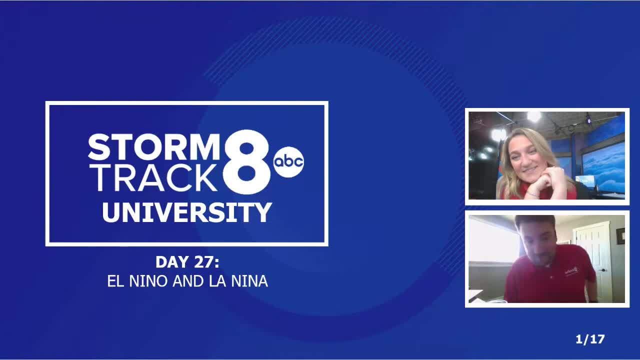 So she can't totally make herself jump over a wall. Andrew and I have gotten the go ahead to come back and we'll be working from home a little bit less, Hopefully, Cooper. Oh yeah, Cooper Can't get too comfortable anymore. 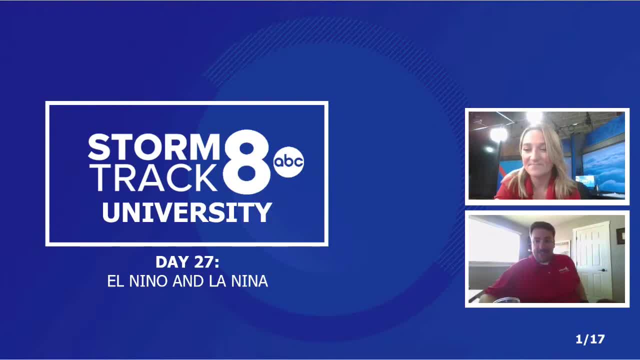 Nope, We're excited, though You look great being back in the studio, even though we've been back in the studio for months on air, but we're back in the studio for not on air days, which is nice- Get to see more people that I haven't seen. 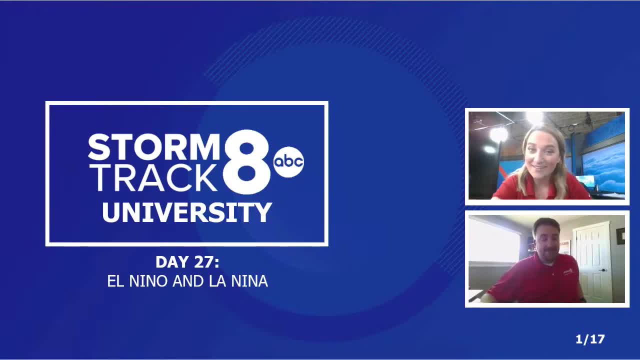 in like over a year. It's crazy. Yeah, it's been a while. I got to see James last Thursday, which was amazing, Isn't that crazy? And I get to see Andrew, and I haven't seen you in person, I think, since we had lunch last summer. 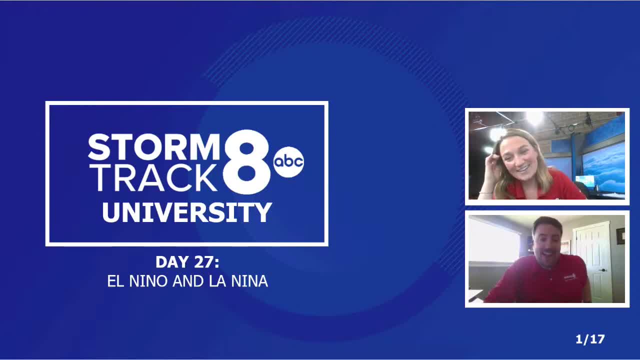 I think that's right. Yeah, it has been that long. literally It's crazy, It is. It's nice to have some normal seat back, though We're getting there, We're turning the corner, I think, finally at this time. 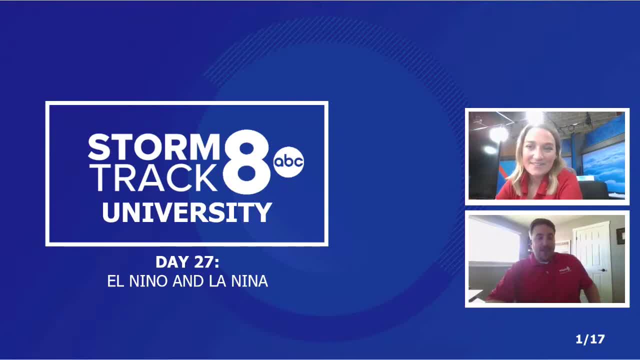 Yes, All right folks, You enjoy the rest of your weekend, Enjoy your Wednesday. I will see you this evening and really the rest of the week until next Tuesday. I think it is during the evening newscast James taking some well-deserved time off. 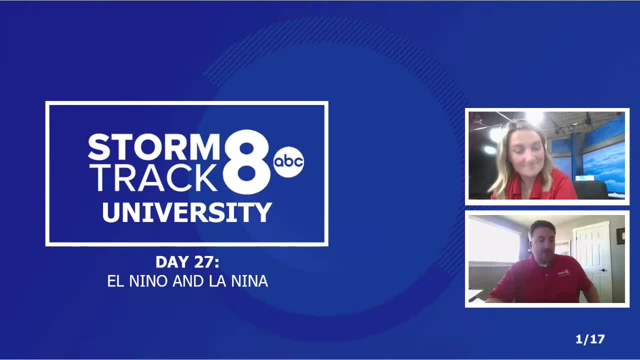 Morgan, we'll see you on Friday, I believe, for GMQC, both editions. So you get the Weekend Warriors taking over the newscast for your Friday, which we have to do. Yes, So we'll see you up and along the way.